Hi, welcome to another video. So this is going to be pretty quick. This is just about finding the intersection of two functions, So I need to tell you how to do that, show you what it is that we're doing, what we're finding, and that you should end with, well, an order pair, Because 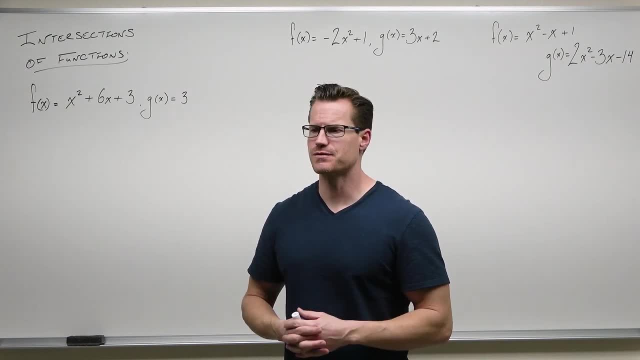 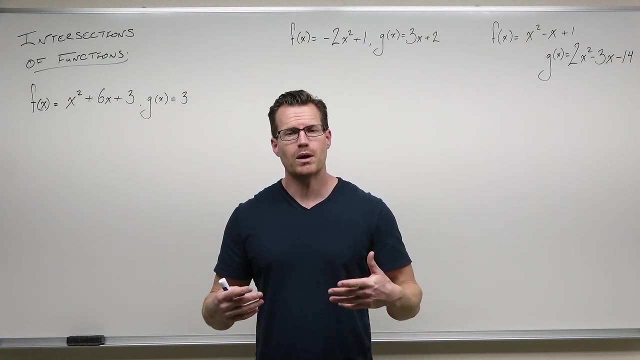 when two functions intersect, we get a point. So that's what we're going to talk about in this video. So we have just three examples. If you're ever asked to find the intersection of two functions, well, what we want to do is set those functions equal. So if the functions are the 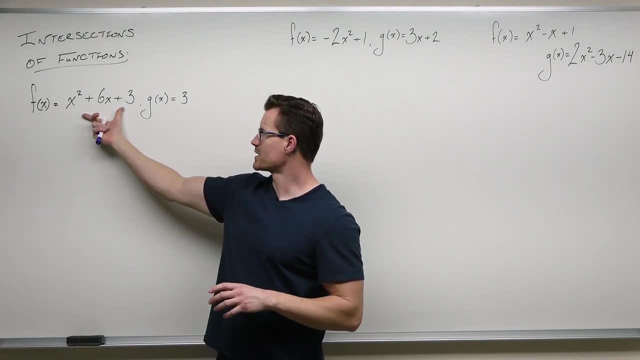 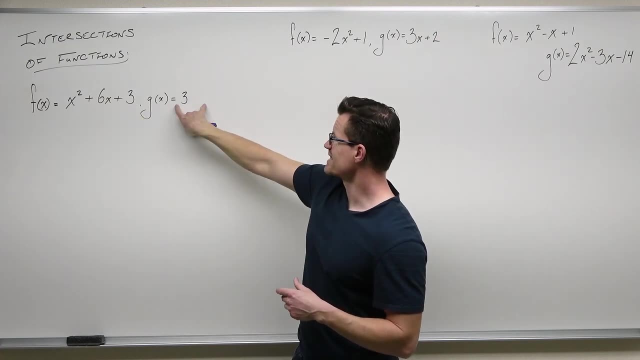 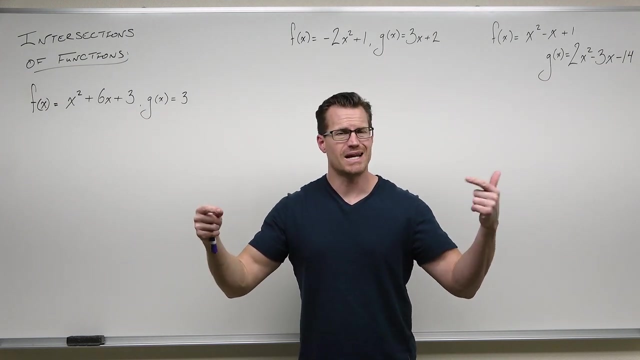 output of some set of some algebraic expression where we plug in a number and get an output if we set our outputs equal. so basically, this gives us an output, this is the output. we set them equal. we find out what x values will it take to get the equal outputs? And by doing 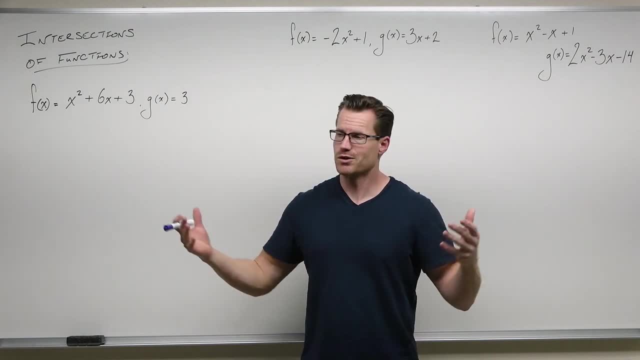 that we find out the points of intersection on two functions. So, in other words, just set them equal. So we're going to say hey, when this function is set equal, we're going to set them equal. So we're going to say hey, when this function is set equal, we're going to set them. 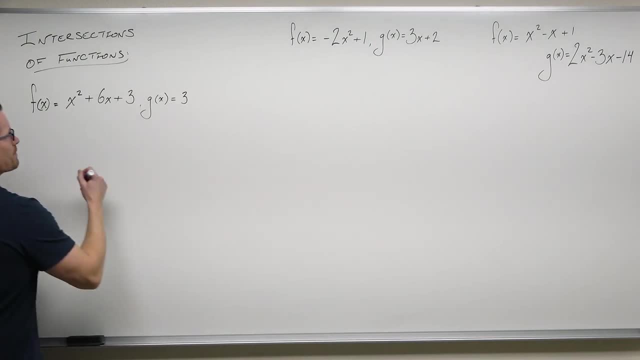 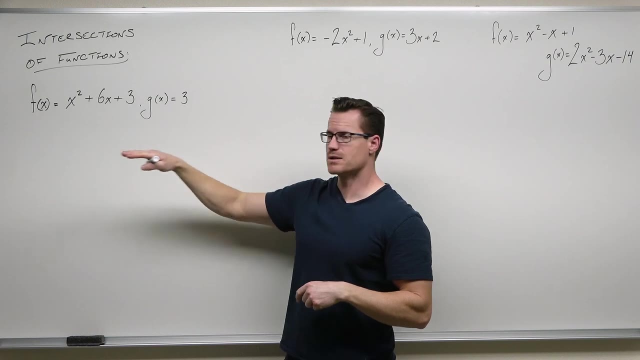 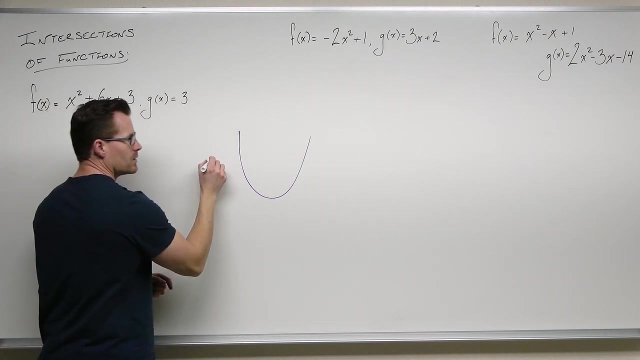 equal. So we do that. Now what we're finding, what this really is, if you think about it, this is a parabola that's upward opening, and this is a constant, which is a horizontal line. So, really, what we're finding on some parabola and some horizontal line, if those things intersect. 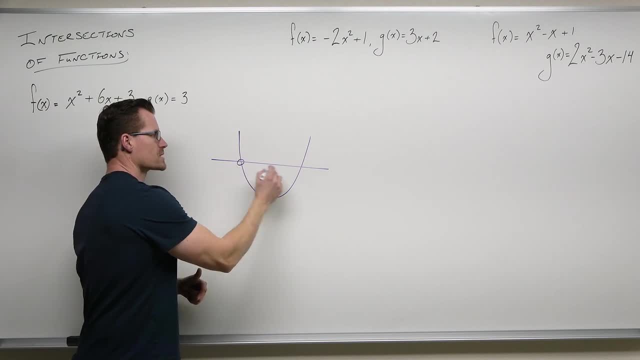 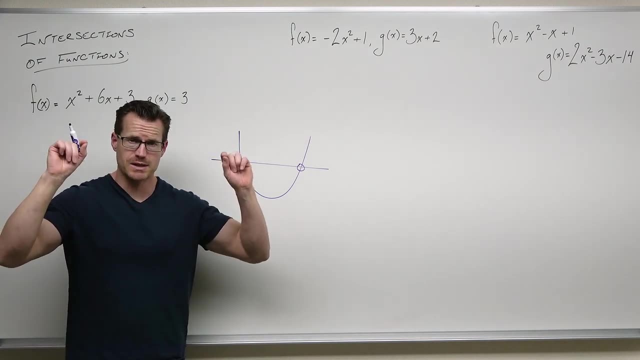 it will be found by setting the functions equal and we'll find the points of intersection at x, comma, y. So we, we set the functions equal, saying hey, we want the y values or outputs to be the same. find the x, this, the x values that give us those equal outputs and that's going to give us the 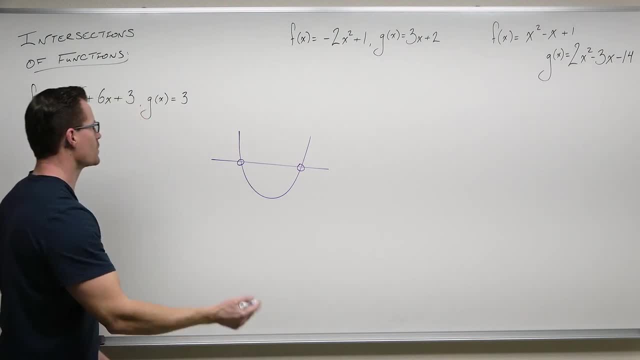 points where the x's are the same and the y's are the same in both of our functions. So when we do that, we're going to see some things that are really familiar. So we're going to see stuff that seems like it's from maybe intermediate algebra. When you set functions equal to one. 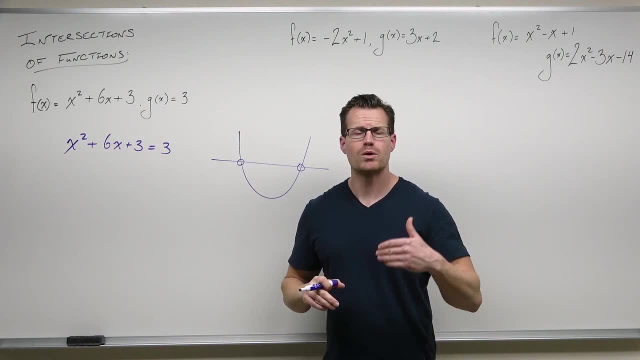 another. you go: oh, what should I? what should I do to solve that? Well, with anything, power two or higher, we're going to see that it's going to be the same. So when we do that, we're going to. 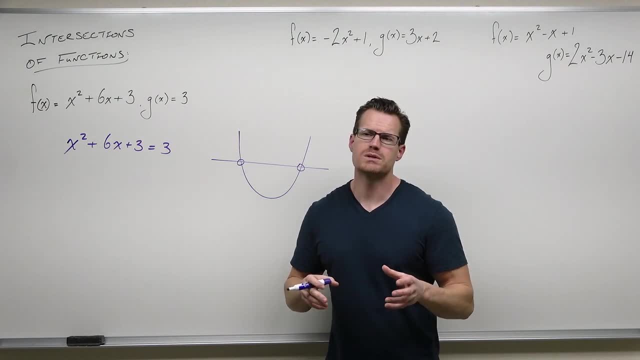 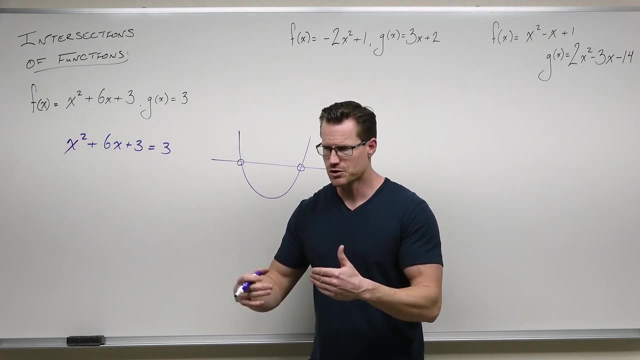 One of the best things we have is factoring or using some of the rational zeros properties we have later on. What we do is we get everything on one side, we get it in order, we get the first term positive- I know this sounds familiar- And then we try to factor it or use the square root. 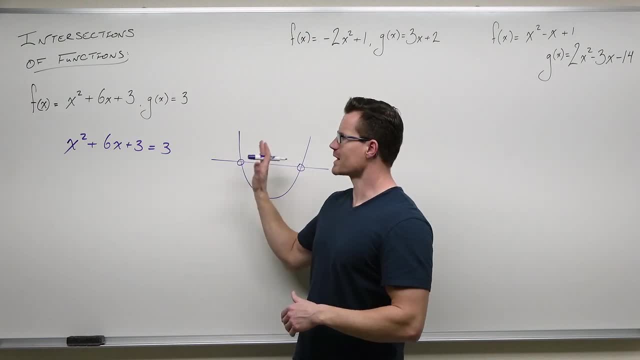 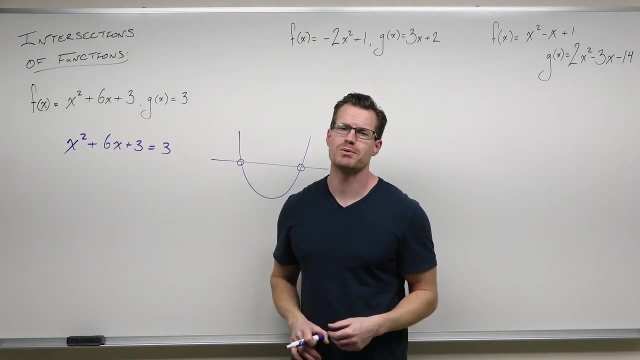 method, Or, if we can't do those things, we do quadratic formula. So we want to get everything on one side in order first term positive and zero on the other side, so that the zero product property works if we can factor it, or quadratic formula works if we can't. So we'd subtract. 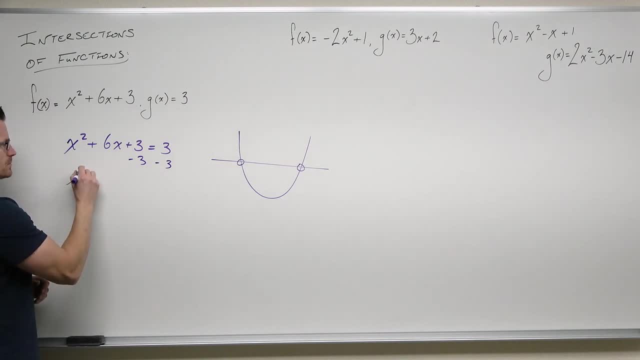 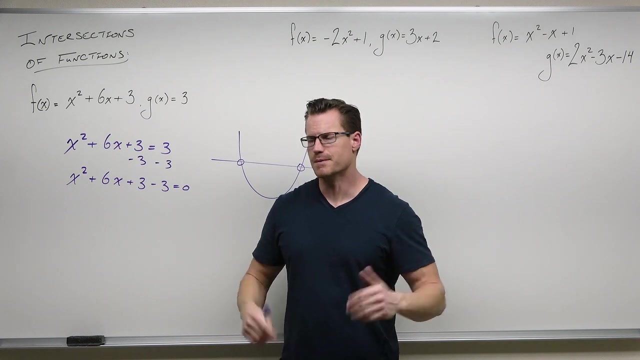 three, And I want you to understand what happens when we do that. I'm going to write this a little funny. I want you to notice. my original parabola is this: x squared plus six, x plus three, It's got a y intercept of three. If I plug in zero, you can see that. Now what happens when I subtract? 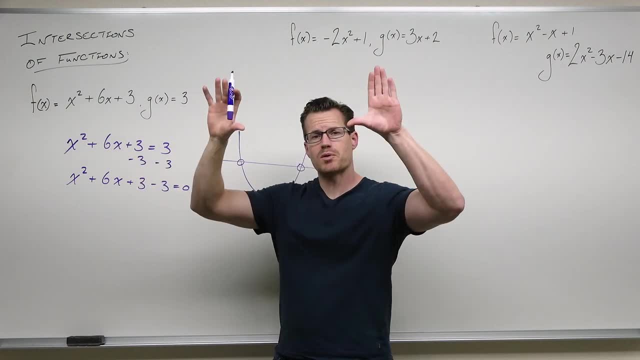 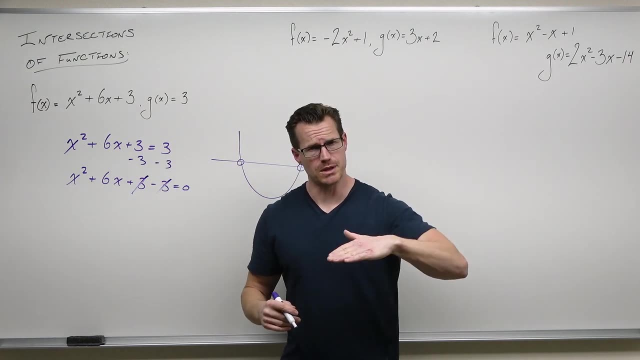 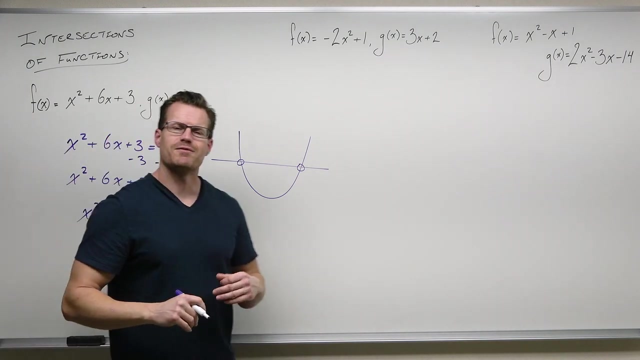 the three, this constant. Basically it shifts this parabola down And it says: all right, if you shift this parabola down, the original parabola subtract three would shift it down three units. By finding the x intercepts of this function, it's like finding the intersection of these two. 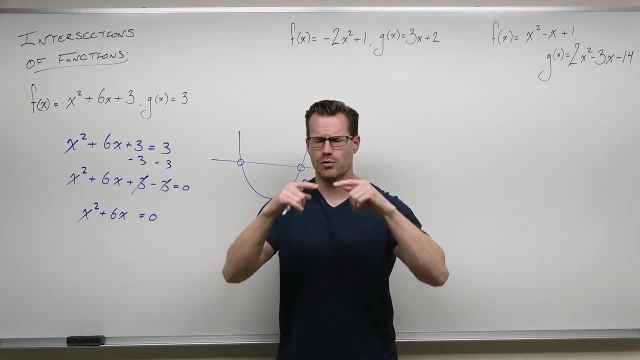 functions. So it's kind of difficult to think of where this parabola crosses the y equals three line or g of x equals three. But if I shift it down three units and think, well, you know what, just shifting this parabola down so that it's kind of sitting on the x-axis, 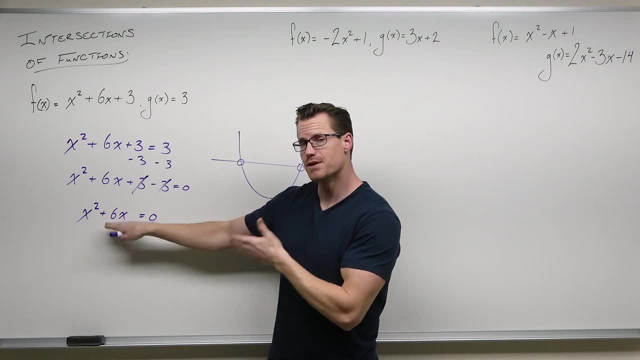 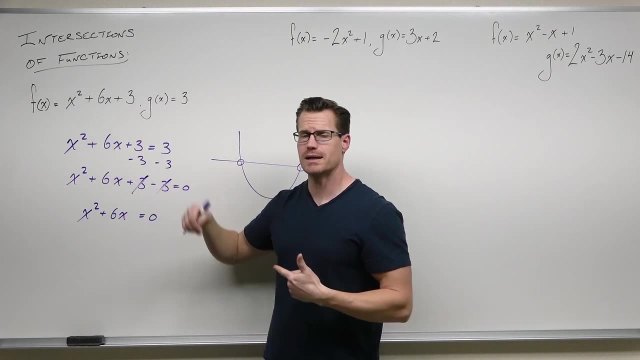 the x-intercepts are very easy to find. So by finding the x-intercepts of this function, we inherently find out the x values where these two functions intersect. The y values- yeah, we'd have to plug in our x's, But this will give us at least the x values where our 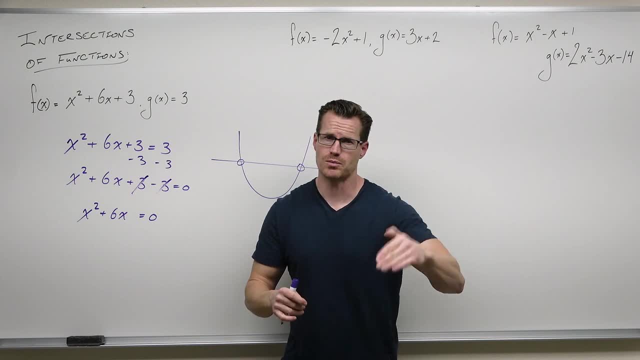 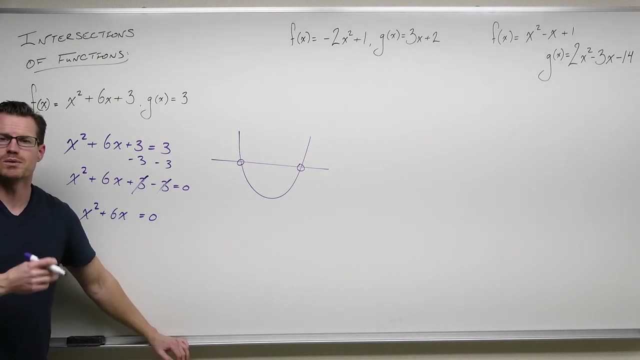 functions are going to intersect, by finding the x-intercepts of a shifted down parabola. Now how we solve it? Number one: we'd always try the square root method And it's not going to work because we can't isolate our power. two, without getting x on the other side. But what we can do? 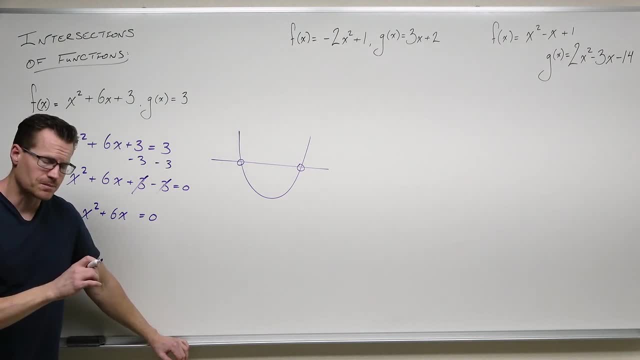 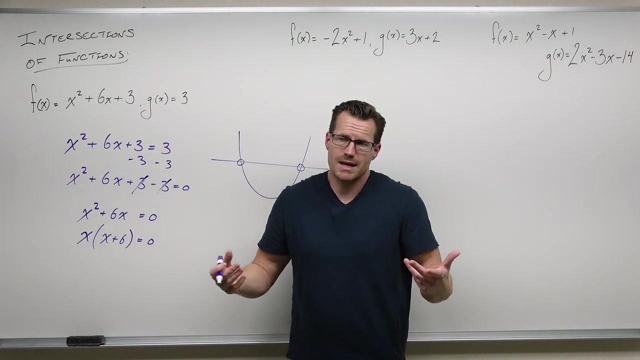 the next step would be: factor Always. factor a GCF. if one exists Here, it does. We factor an x And because we got everything on one side, we have a zero on the right-hand side. the zero product property works. It says: yeah. 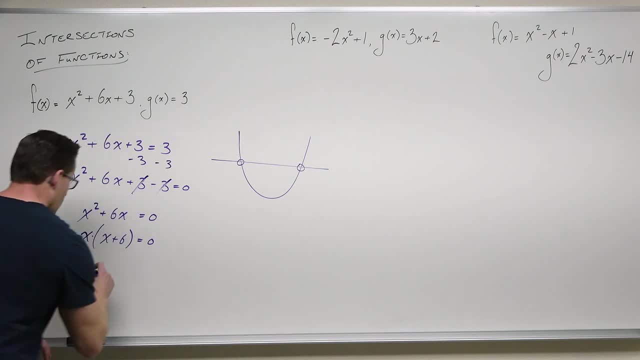 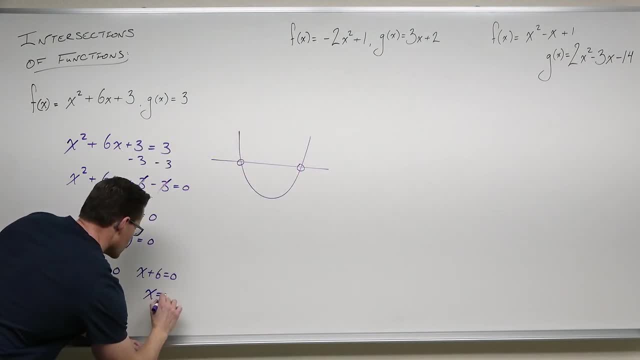 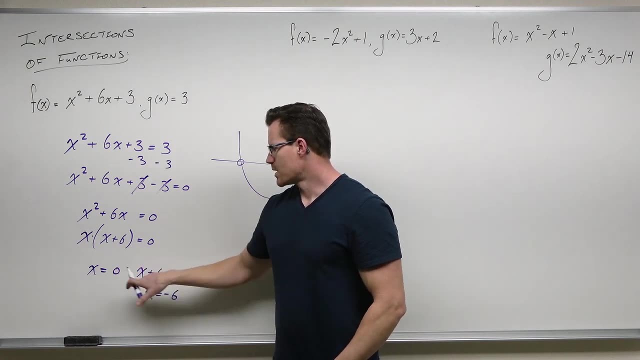 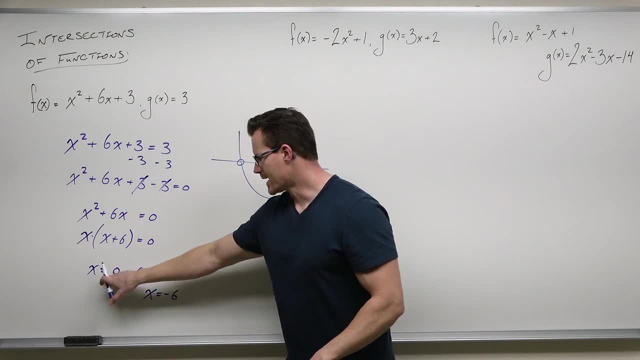 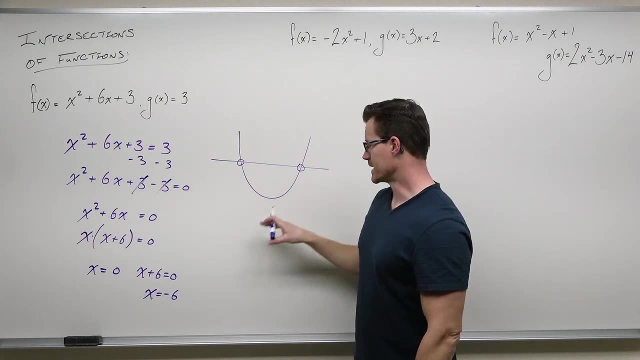 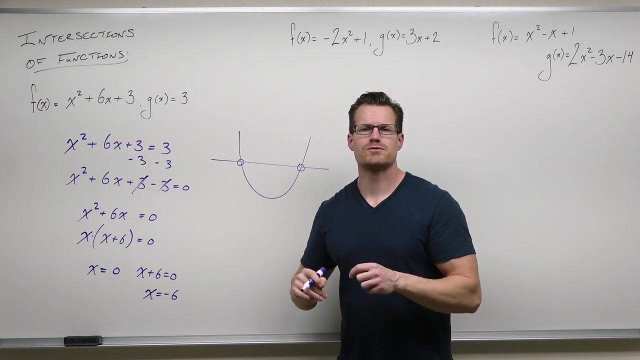 zero. But what it also represents is the x values where this function and this function intersect. So this will intersect at x equals zero and x equals negative six. What we want to do is go a little bit further. We want to take those values and find the ordered. 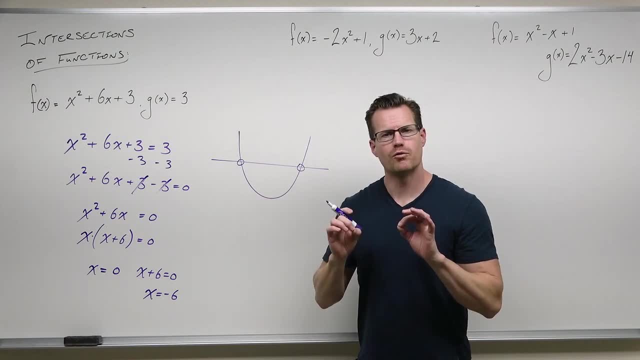 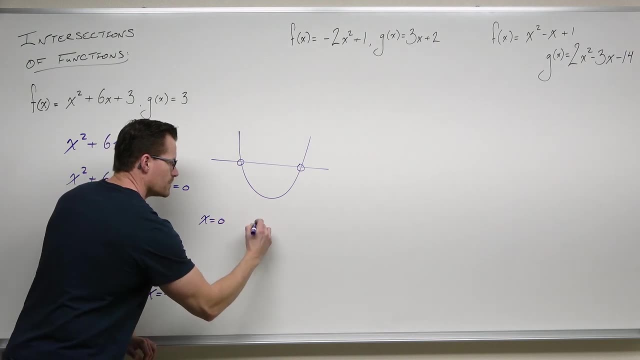 pairs of intersection where the points. you're trying to find the point here of where these two graphs intersect. So what we're going to do is say you know what, from the x equals zero and x equals negative six. we should be able to plug those into one of our functions. 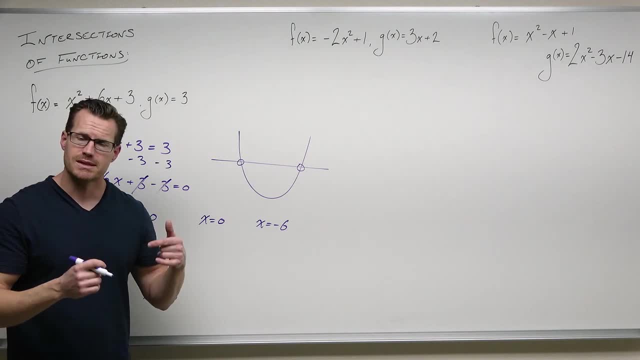 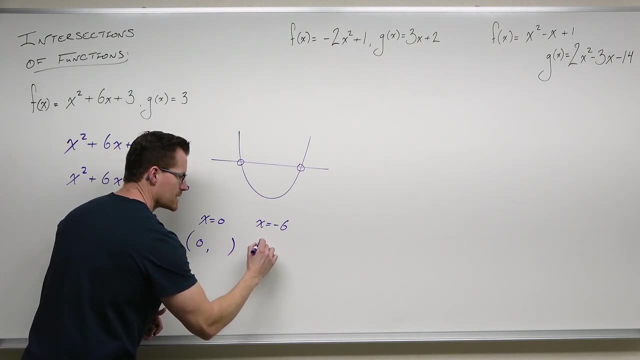 or both of our functions, if you actually want to check your work and see that this actually gives us what we want. So we're going to create an ordered pair: zero comma- some number- and negative six comma- some number, because that will be our points at intersection. 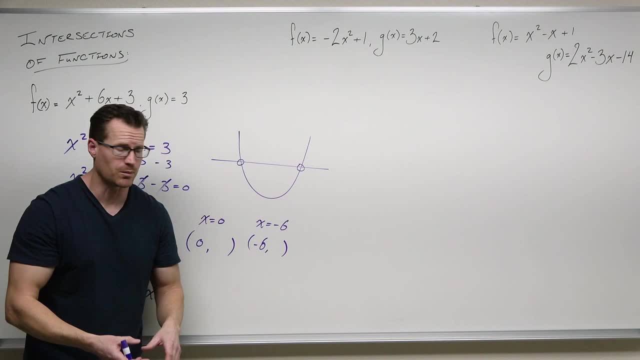 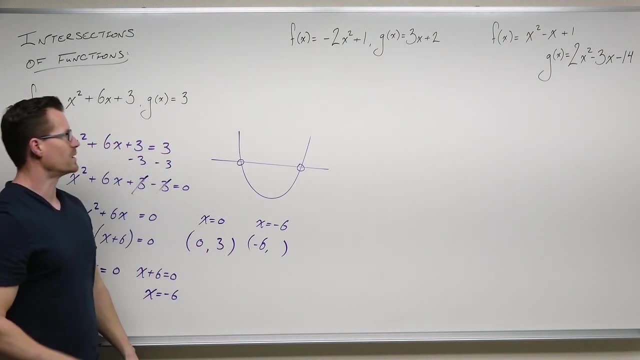 from our graph stemming from the fact that we found the x intercepts from a shifted down parabola. If we plug in zero here, we get zero. squared plus six times zero. zero plus three is three. You know, wait a minute, Can't I just plug in zero here and get three? Yeah, that's the whole. 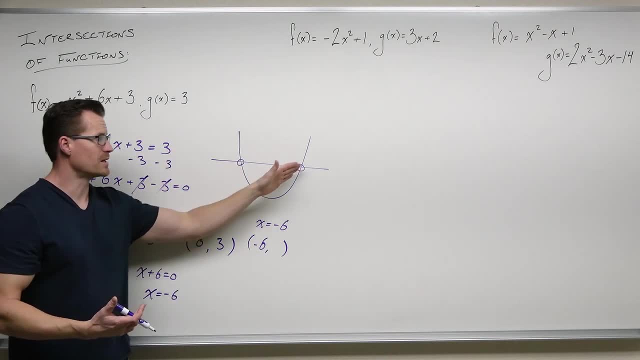 point. right, That's a constant. So where this parabola would intersect, this constant of three would have to be at a y value of three. In fact we could just put three here. We know it's going to intersect at something. comma three, because that's the only. 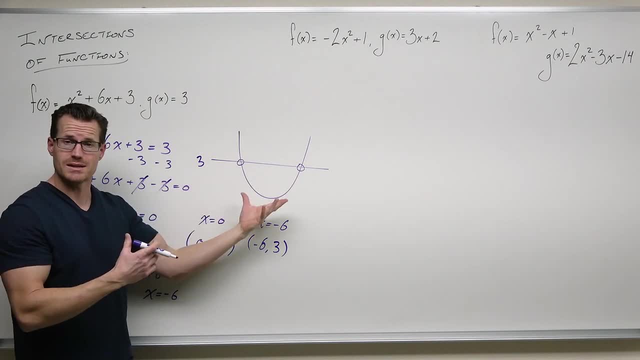 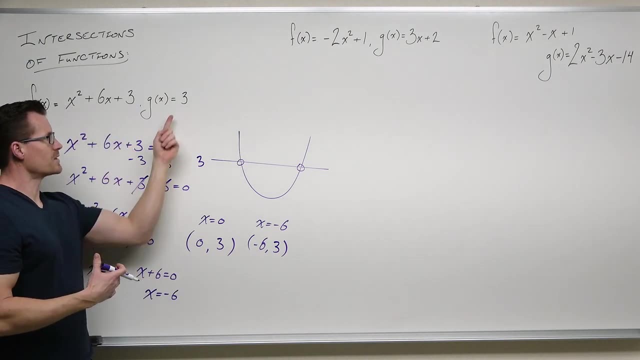 place a horizontal line. that's, the only output of a horizontal line is three in this case. Now what I did, though, is I checked my work, So I plugged in zero and said: all right, zero plus zero plus three is three. This is also three. That's how you check your work to make. 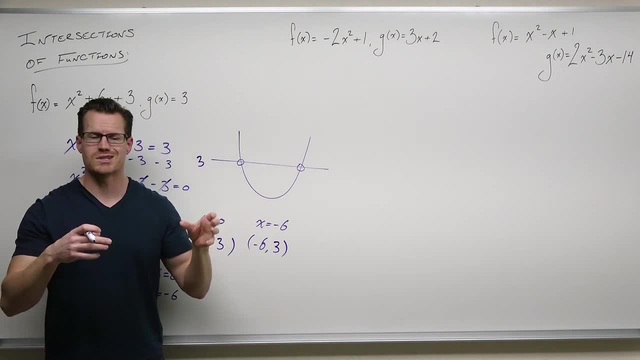 sure you have the correct intersection. Plug in your x value to both functions and it needs to be the same. That tells you that that one x value gives you the same output on both functions. That has to be a common point. So we're going to plug in zero and we're going to plug in three. 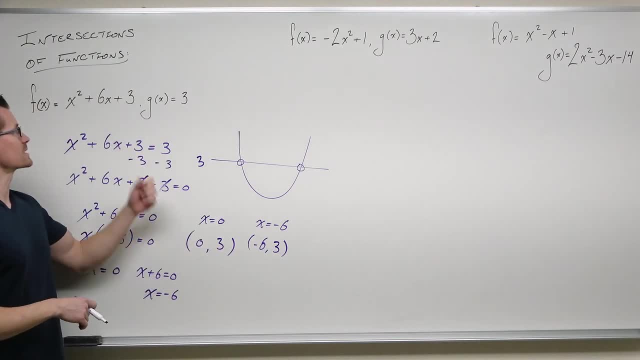 That's the point between the two and therefore an intersection. Try negative six, Negative six squared is positive 36.. Six times negative six is negative 36.. 36 plus negative. 36 plus three is three. Also, we plug in here. Well, there's no place to plug it in. That's why it's called. 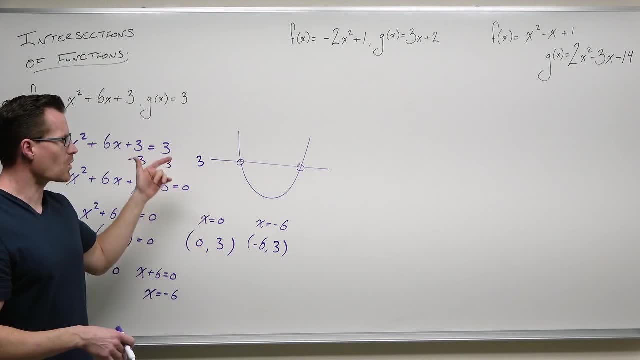 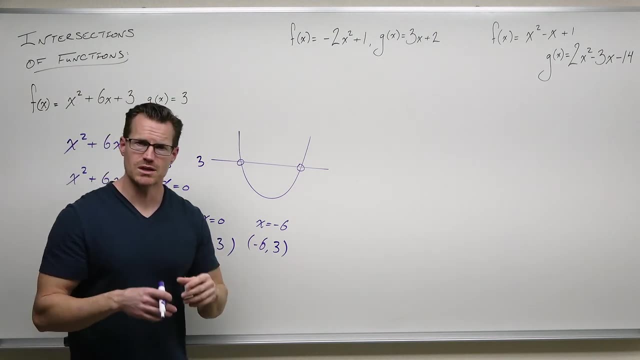 constant and you get three. So we know that these two points are the two points of intersection of this parabola and that horizontal line. That's what we are doing when we're setting two functions. equal is refining the points of intersection. That's how you do it. 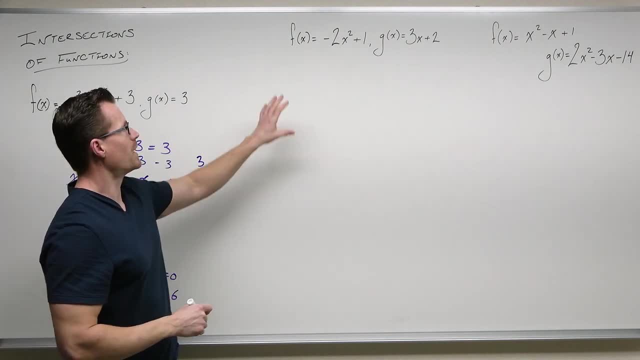 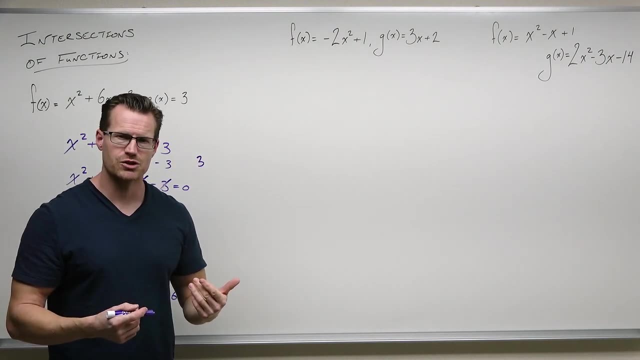 Okay, let's move on a little bit. We have two other functions here. We've got f of x equals negative two x squared plus one. We've got g of x equals three x plus two. Before we go and find the intersection, I want to understand what we're doing. You need to know what that shape, sort of. 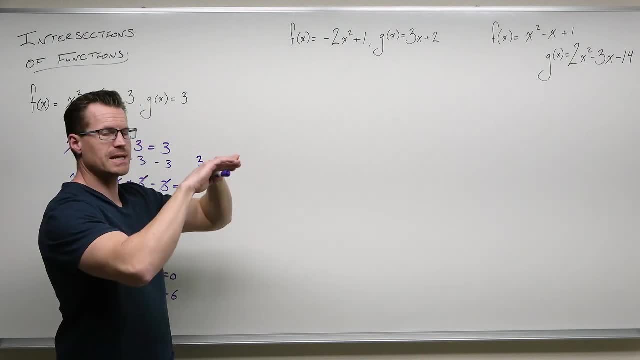 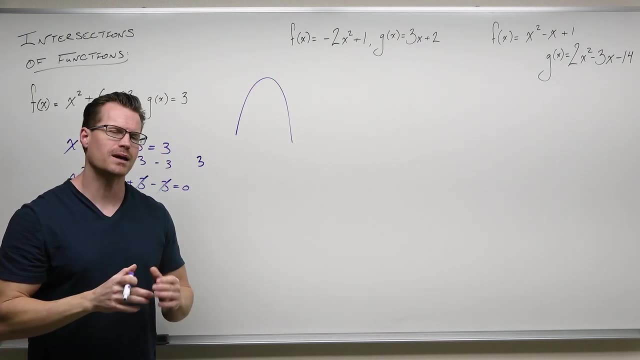 looks like You need to recognize. it is a parabola. It's power two, but it's a downward opening. So this graph looks like this Somewhere on an xy coordinate plane. I don't really care. right now We're going to find the points of intersection, but I just want to get the picture in your head. 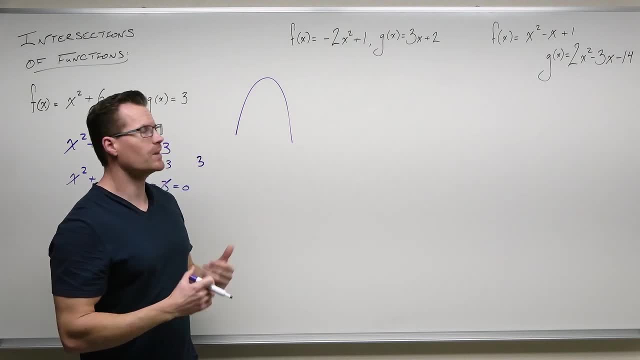 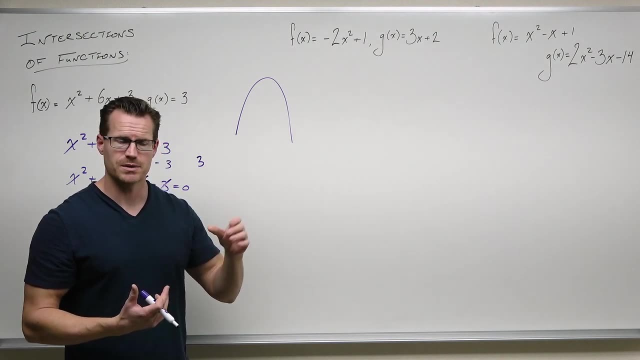 of what you're doing, This function. is that a parabola? Well, no, it doesn't have a power two. What it does have is a slope and y-intercept. This is in slope-intercept form. It has a y-intercept of two. It's got a. 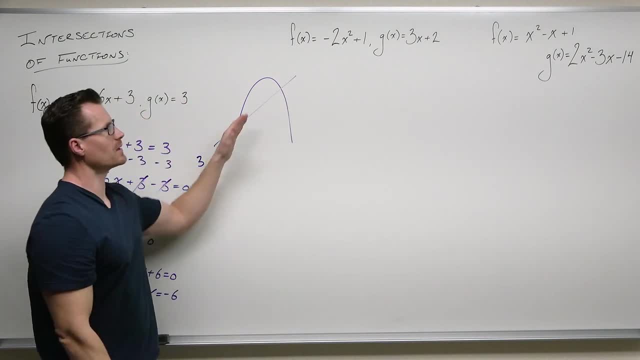 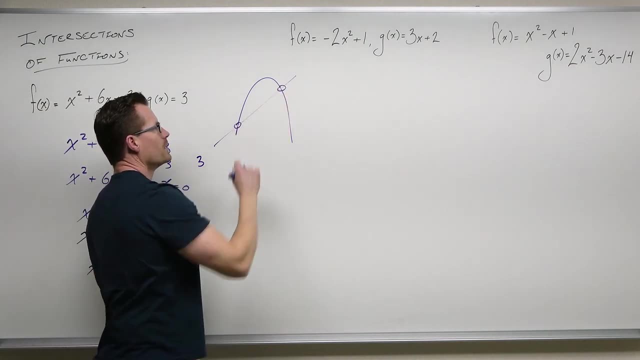 slope of three. So this is some sort of climbing functions. climbing line: It's a line because it has a slope, and y-intercept It's in that linear equation form. If this intersects, that's about where it's going to be. So we're going to intersect this downward opening. We're going to intersect. 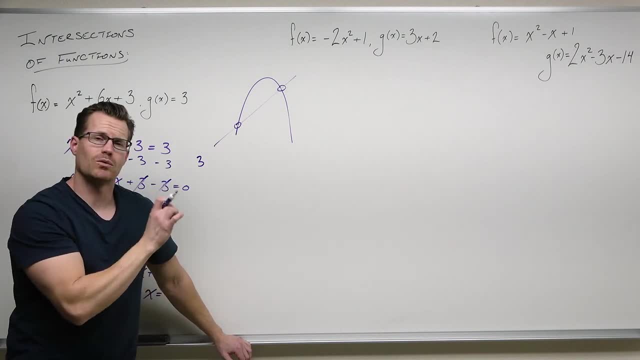 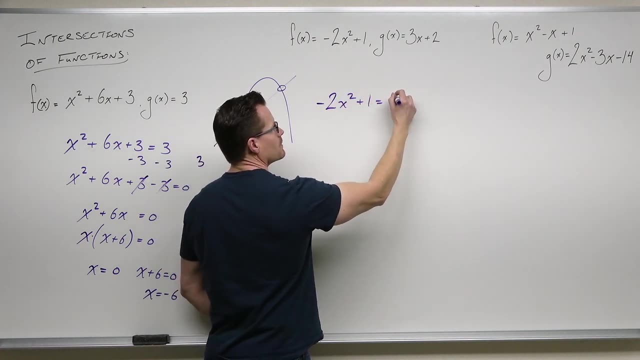 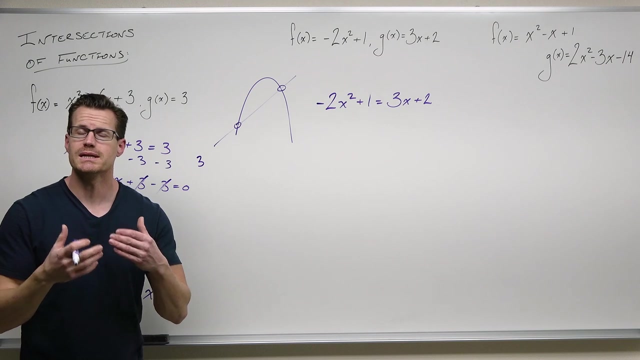 this downward opening parabola with some sort of a line, And that's exactly what we're finding. How to find, that is, set the functions equal, So we'd have negative. two x squared plus one equals three x plus two. From here, man, we don't need to keep the same nature of what these are. I. 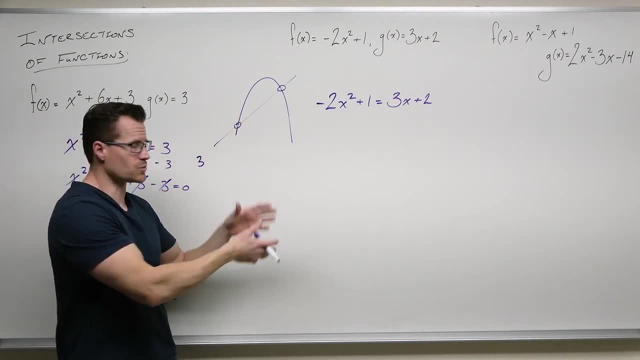 don't really care that. it's a parabola and a line. This is what you're finding, This is what you're going to know when you solve this, But how to solve it doesn't care about keeping these forms In order to solve this. 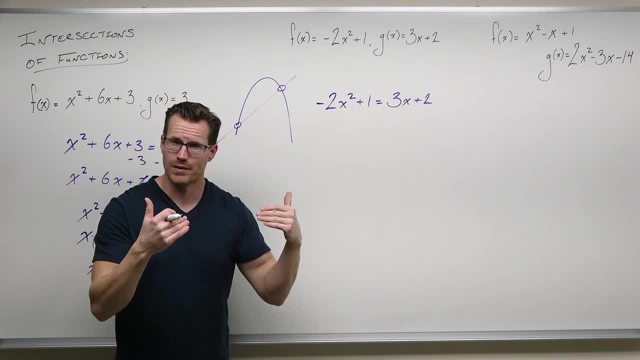 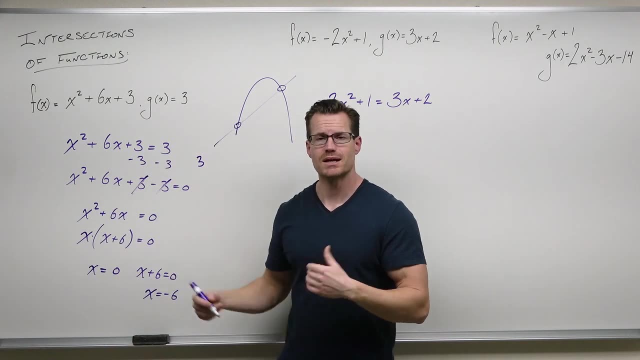 we're basically going to change this to a different parabola, Find out where that parabola crosses the x-axis, And then those x-intercepts are going to represent the x-coordinates of the points, like we did in the previous example. So what I mean by all that is man, just do the same. 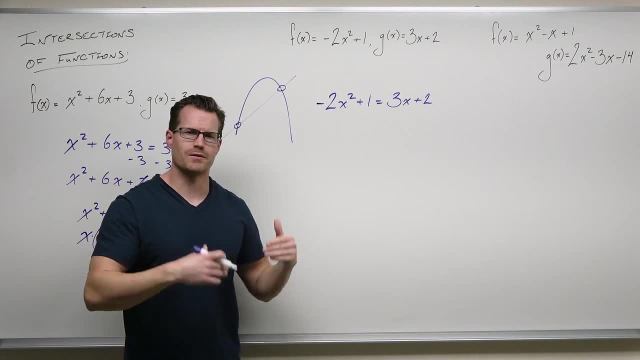 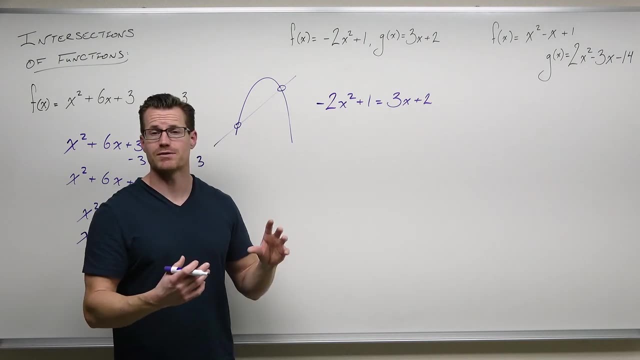 thing we've been doing. Let's get everything on one side, Let's get it in order, Let's get the first term positive. Let's see if the squared method works. If not, let's see if we can factor. If so, great do it. We're going to be able to factor this. If not, we use the quadratic formula. 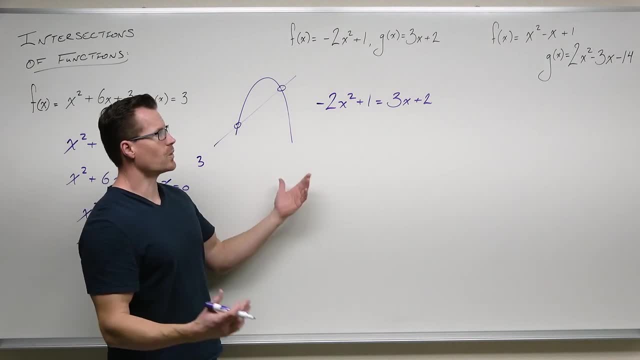 But in all those cases, you want zero on one side. Now what's the appropriate choice? Should we move the stuff from the right to the left, or the stuff from the left to the right? Well, it seems better to move the things from the left to. 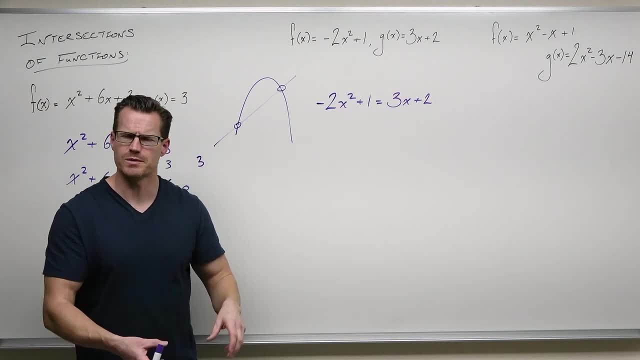 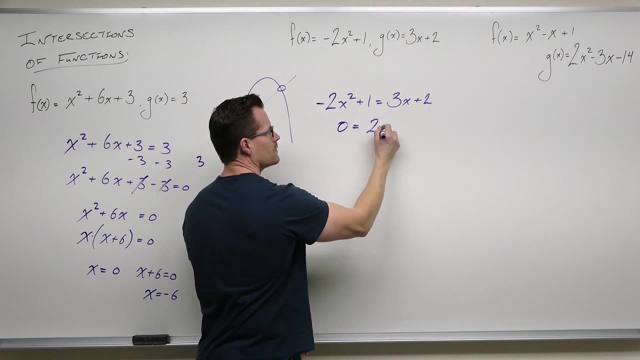 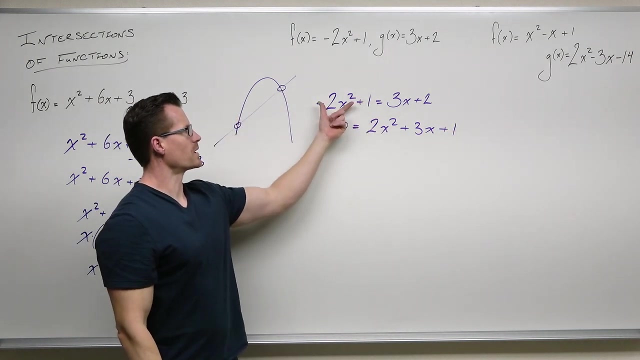 the right so that our first term becomes positive. We want the x-squared term to be the first term because it has the largest power. So if we add 2x squared and we subtract 1.. So adding 2x squared, we get 2x squared. Subtracting 1, we get 1.. 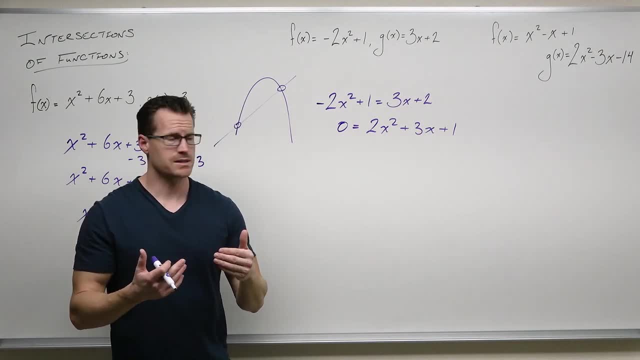 Now we have to do something else. We have to do something else. We have to do something else. We have this setup to look like a different parabola. Yes, this is an upward opening parabola. It's set equal to zero. It's finding x-intercepts, But because we set this equal, 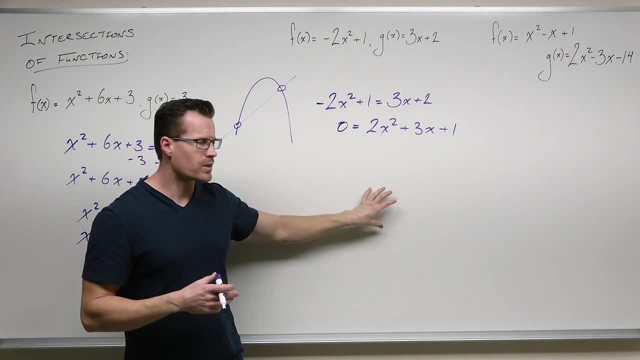 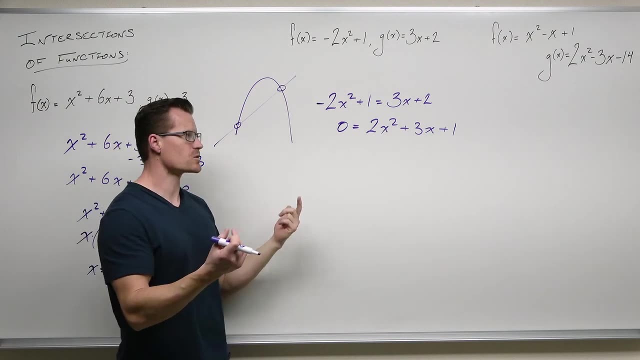 this stemmed from this idea. the x's we get here, even though they represent x-intercepts for this function, they'll represent intersection values of x for these two functions. So we solve it the same exact way: Squared method not going to work. Factoring: yeah, the factoring is going to work. 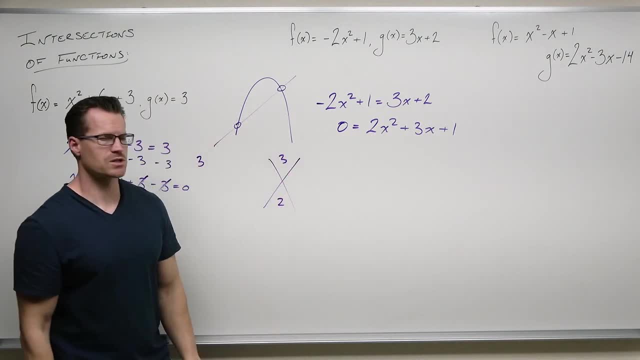 We know that we'd have 3 and 2 times 1 gives us 2.. We're adding to 3, we're multiplying to 2. They both have to be positive. They have to be 2 and 1.. So that adds. 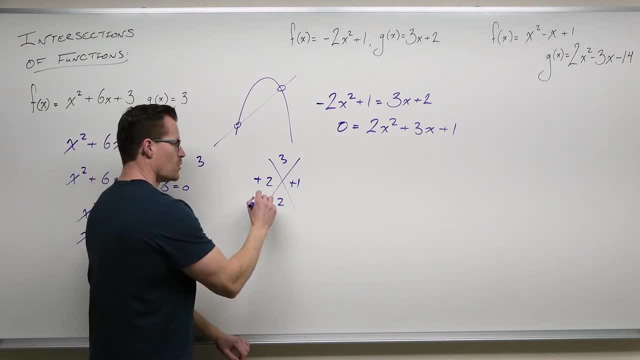 to 3 and multiplies to 2.. I love the shortcut for this. At this point in our factoring lives, we can use pretty much anything we want. I like doing the shortcut and simplifying. I showed this to you in another video. One factor here will be: look at your denominator. 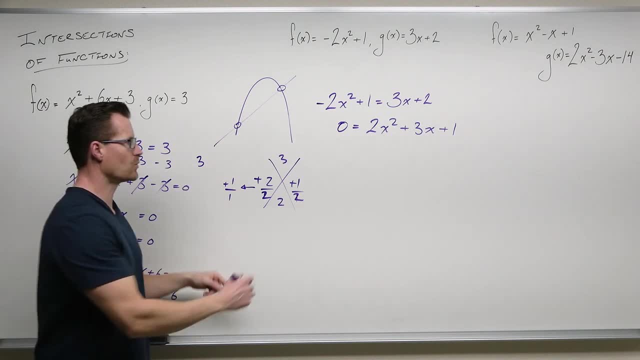 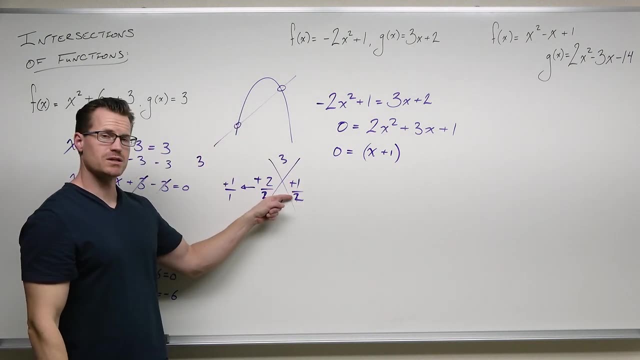 Your denominator says one factor will have 1x and then you'll add 1.. This fraction says denominator says you'll have two x's in one factor and you'll add 1.. Also, we learned that if we just change these signs, it will give us our x values. 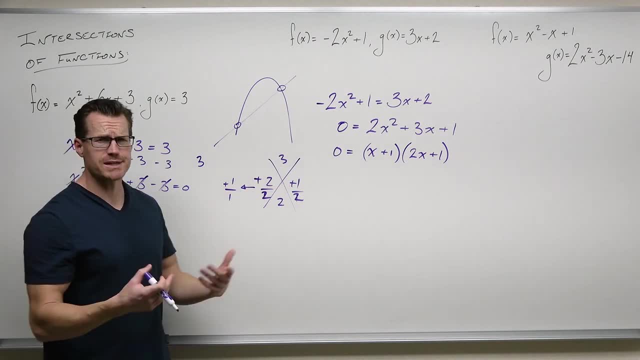 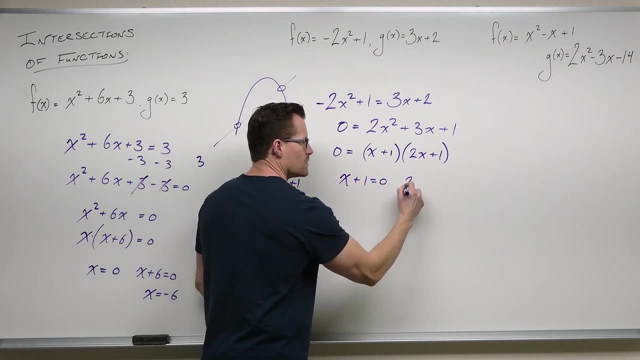 You can do that too. The factoring itself isn't really valuable for us right now, It's just getting us those x values of our intersection points. So by the zero-product property we can set these equal to zero. We'll subtract 1.. We'll subtract 1 and add. 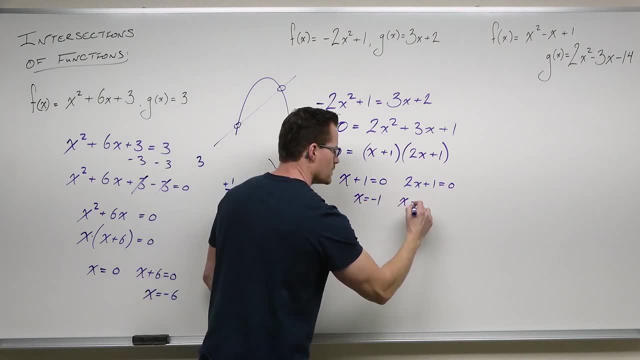 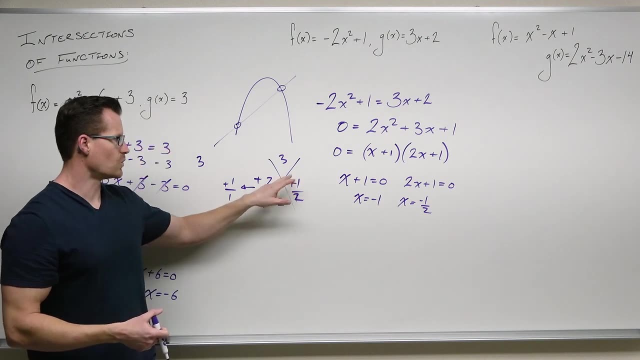 and divide by 2. And we notice that's exactly what we get here. This is the value 1.. If I change the sign, that's negative 1.. Here's 1 half. Change the sign That's negative 1 half. That's great We. 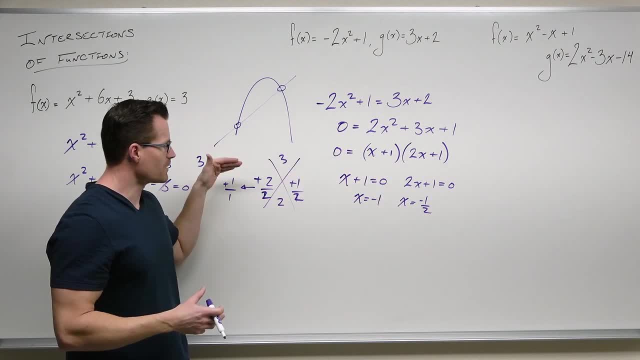 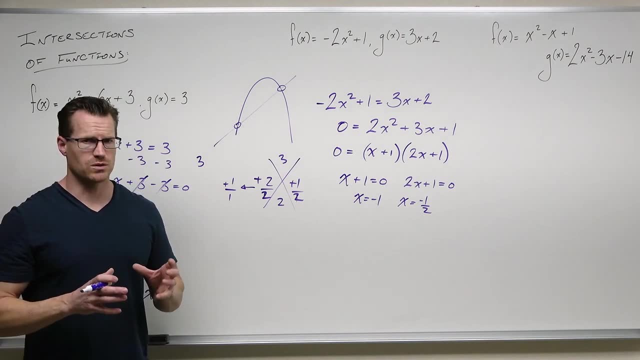 can totally do that. If you don't need to show your factoring, you can go directly from here to the x values of your points of intersection. Now, there is one thing that we want to make sure that we do: We don't want to leave it just as x values Whenever you're finding intersections. 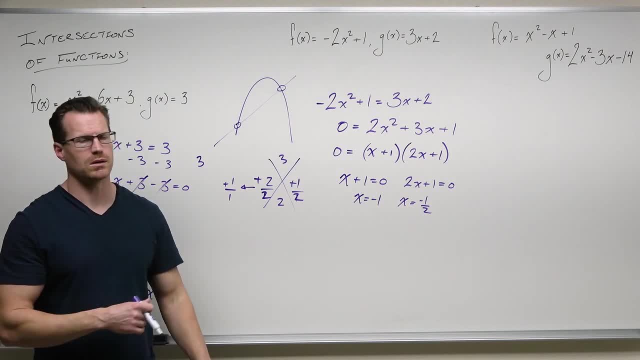 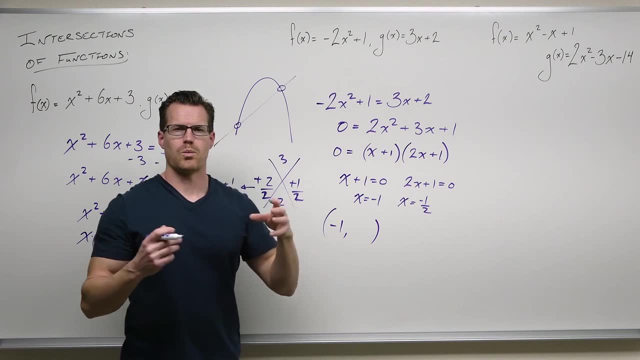 we want to leave them as points. We want to get the point here. So to do that, I'm going to plug in negative 1. I'm going to do it to both of my functions. Why Is that necessary? No, but it's. 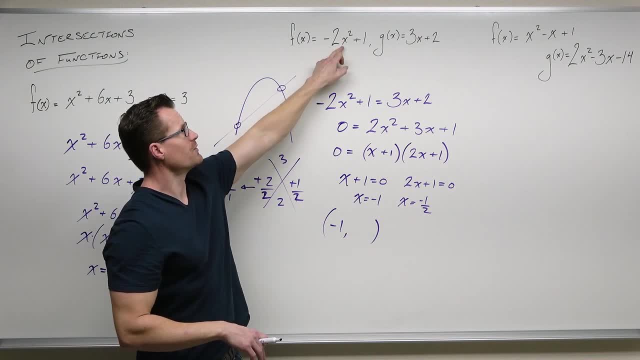 a good idea so that we can check our work. So if I plug in negative 1, negative 1, squared is positive 1. Positive 1 times negative 2 is going to give us negative 2. Negative 2 plus 1 is: 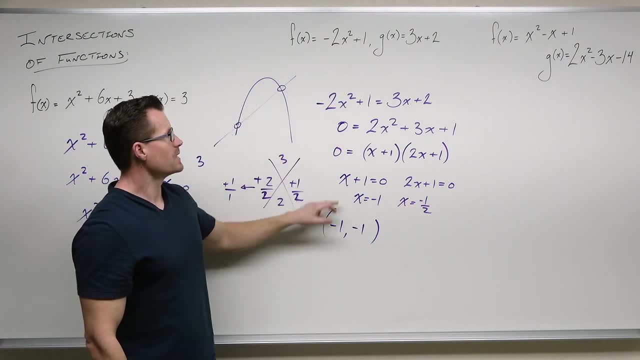 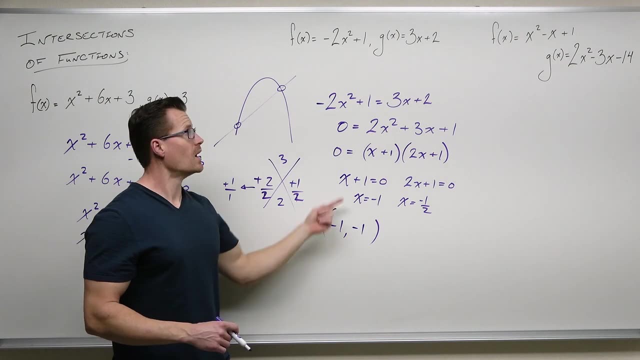 negative 1.. If I take negative 1, same value, plug it in here. 3 times negative. 1 is negative. 3 plus 2 is negative 1.. So I took this 1 x value. I plugged it into both of my functions just to make sure that that gave me the same. 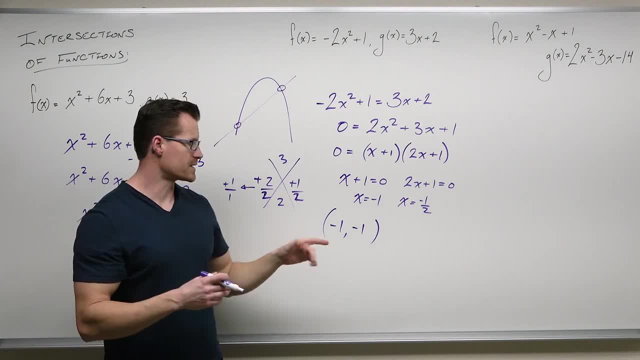 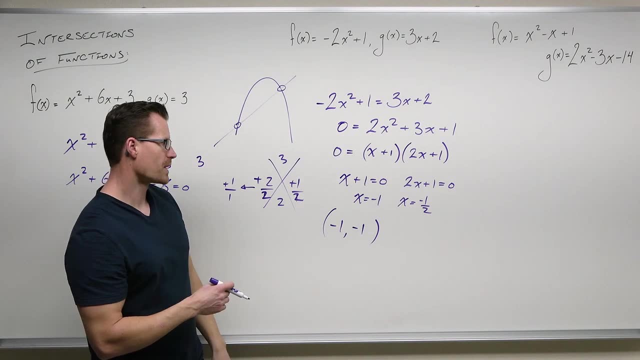 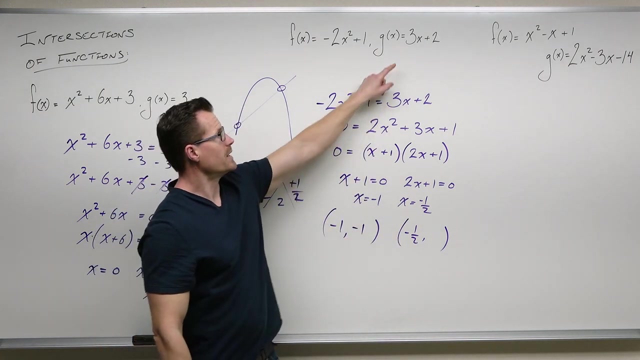 output That totally verifies that this is a point of intersection for both of our functions. So this looks like this point on our graph: Let's plug in negative 1 half. If we plug in negative 1 half, negative 1 half to both. 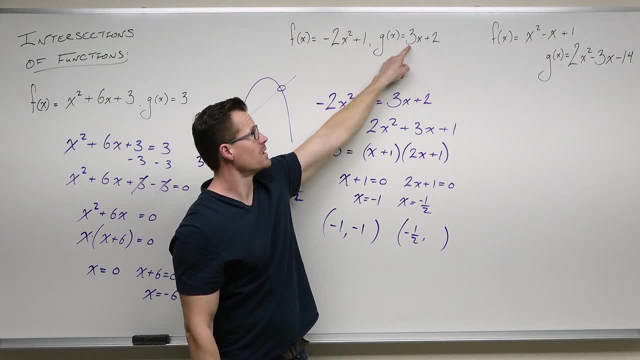 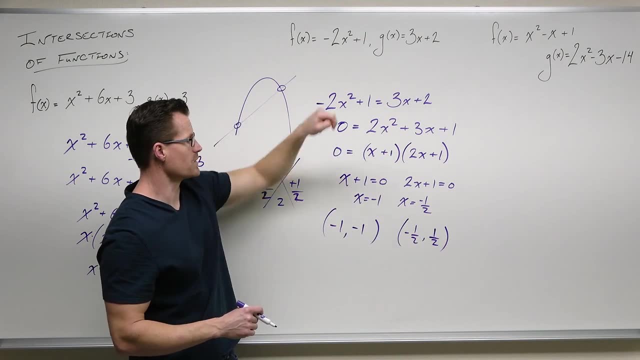 our functions. negative 1 half times 3 is negative 3 halves plus 2 is positive 1 half. Now we better get the same thing if we plug in negative 1 half to our x value here Negative 1 half squared is: 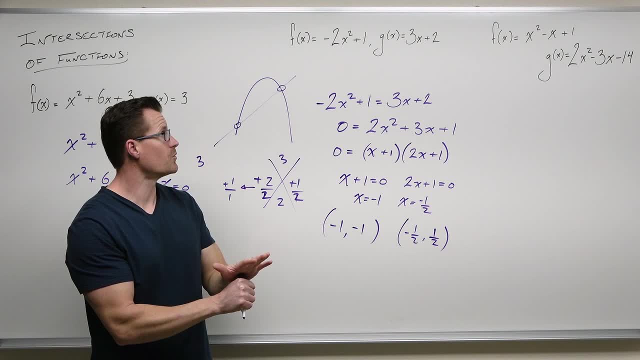 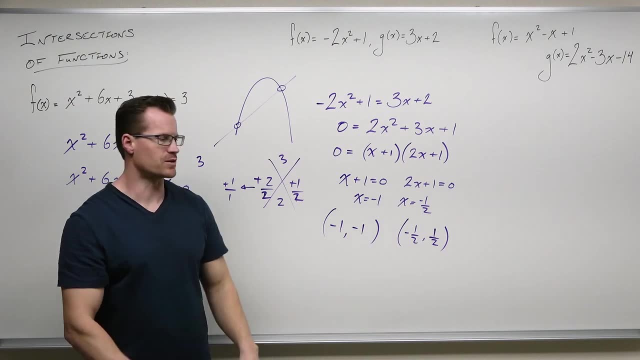 positive 1 fourth, 1 fourth times negative. 2 is negative 1 half plus 1 is positive 1 half. So we know that this value, plugged into both of our functions, gives us 1 half. That's the other point of intersection. So let's see That would look something like. 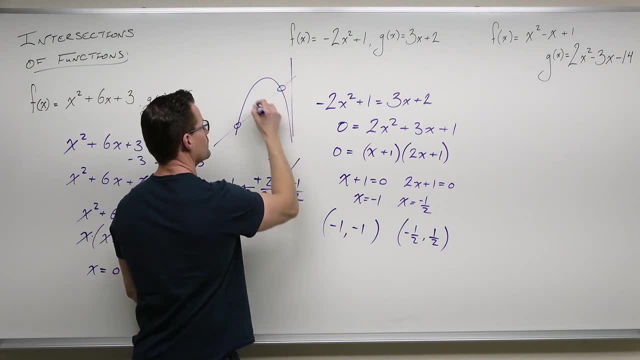 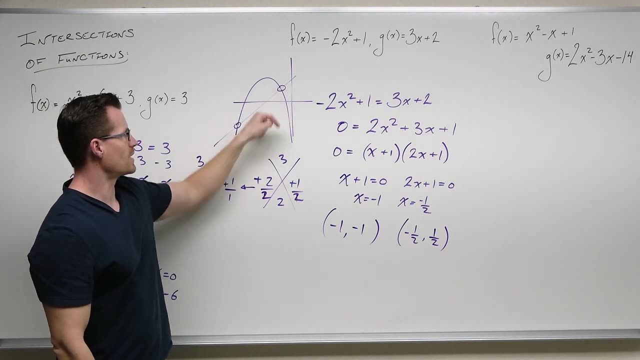 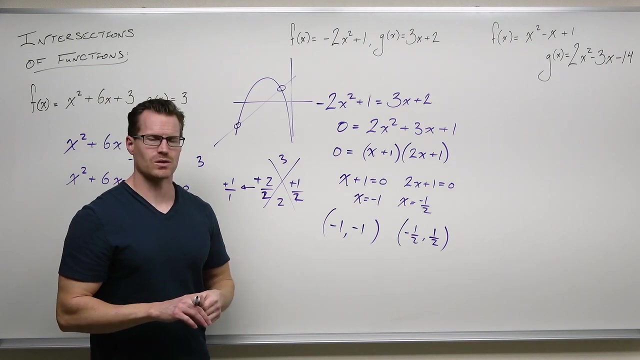 this Scale's a little off, but plug in negative 1, get out negative 1, plug in negative 1 half, get out positive 1 half. That's about where that function crosses the other function, where those two functions intersect. The x and y actors aren't exactly right. I'm just kind of showing you a very 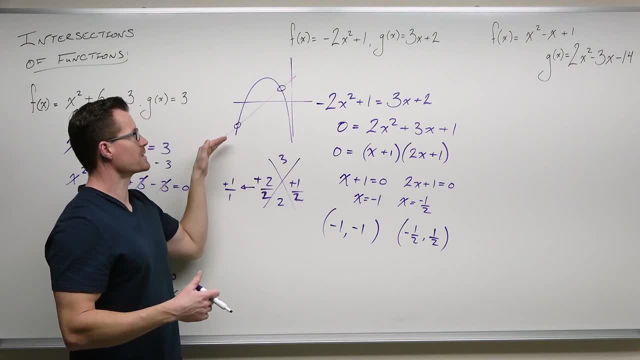 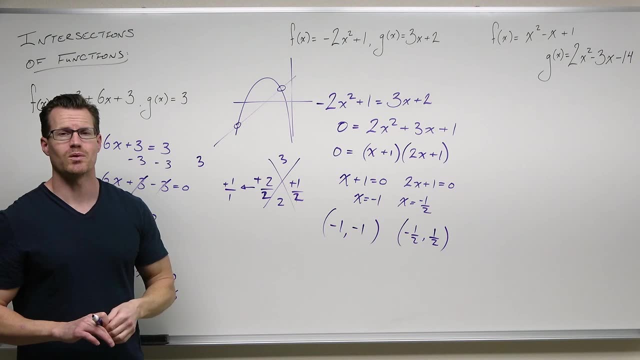 loose visual interpretation of what's going on. That's the downward opening parabola. This is that positive sloped line and we're finding where those things cross, doing it kind of a cool way. So let's come back. We'll do one more example. All right, last one, And again what we've got. 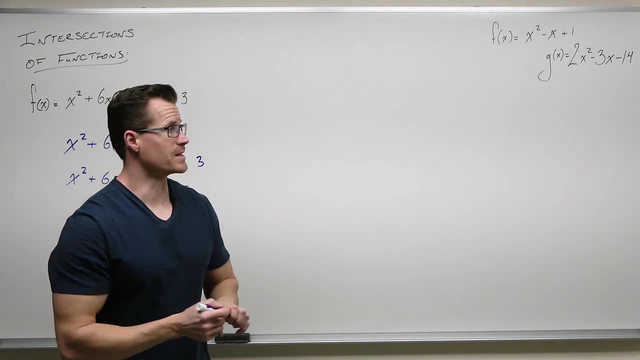 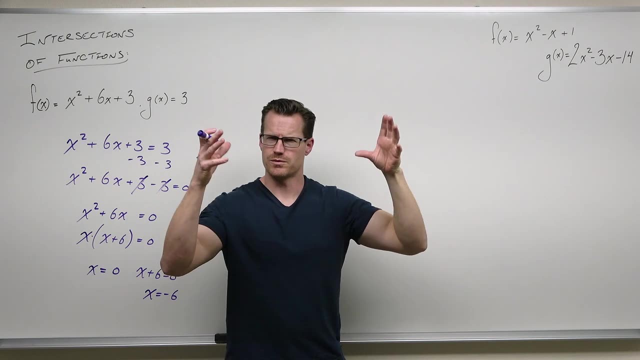 here we have two parabolas and we're trying to see where those things intersect. One of them is upward opening, but a little bit stretched. A vertical stretch is going to be narrow. One of them is a normal sort of parabola, not vertically stretched at all. So we have one. 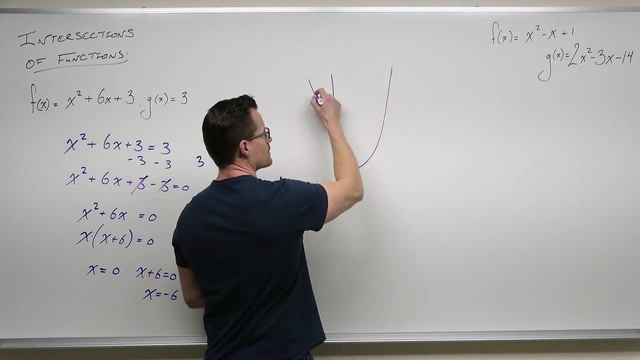 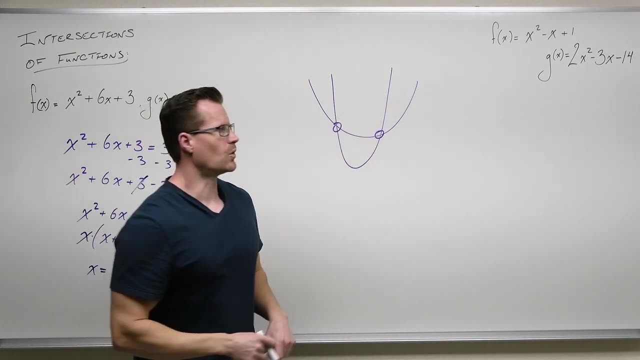 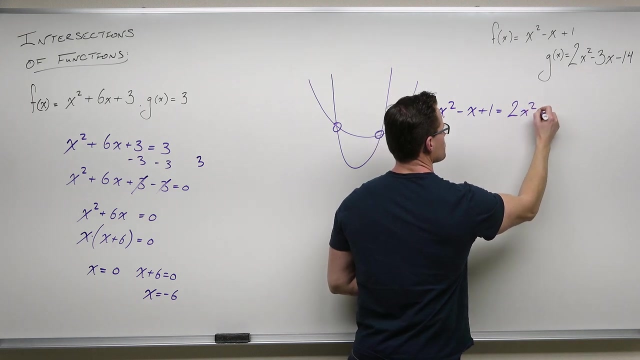 like this and one like that, And we're going to find out these two points of intersection. How we do that is we're going to go to the next step, which is to find the moving points. So we're do it every time, Just set them equal, And we're going to go through the same process we do for. 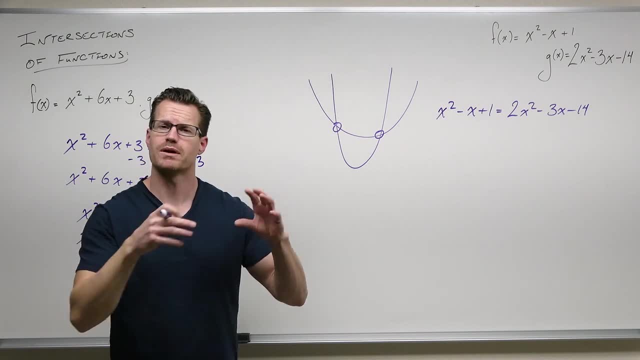 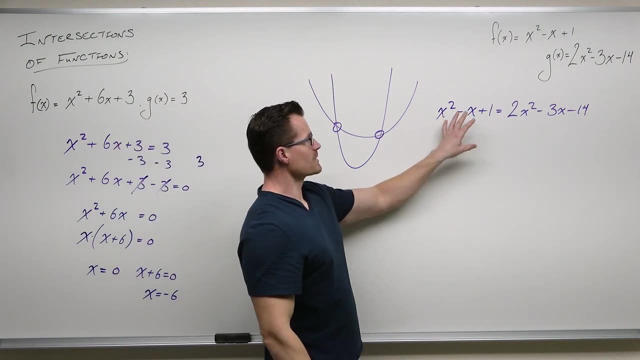 solving for every single thing that has a power 2 or more. We're going to get everything on one side in order, first term positive and see if we can square method factor or quadratic formula if we have quadratics. So let's get the stuff from the left moved over to the right by adding: 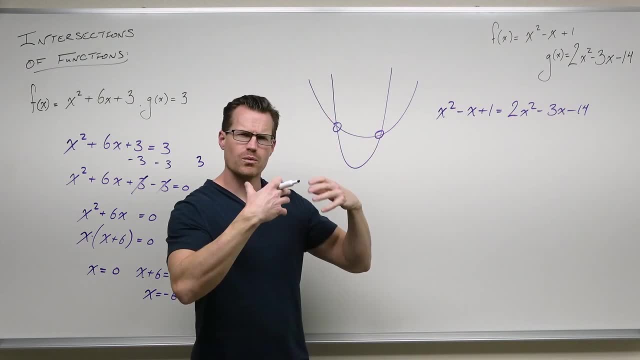 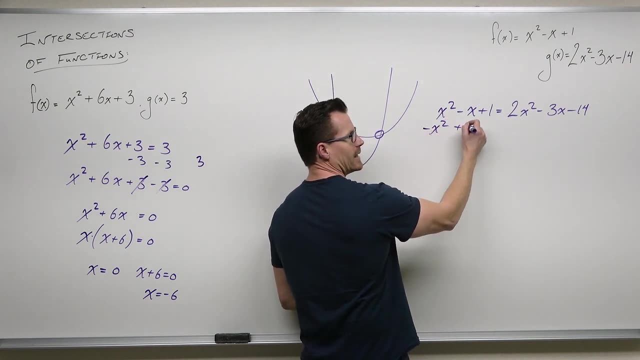 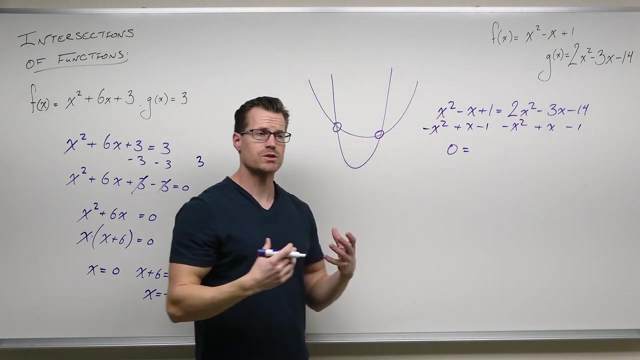 or subtracting respectively, Because that has a larger coefficient. we're going to do that. We don't want to move this over here, or first term would be negative. So we're going to subtract x squared, add x and subtract 1.. That of course gives us a 0, which is really nice if factoring. 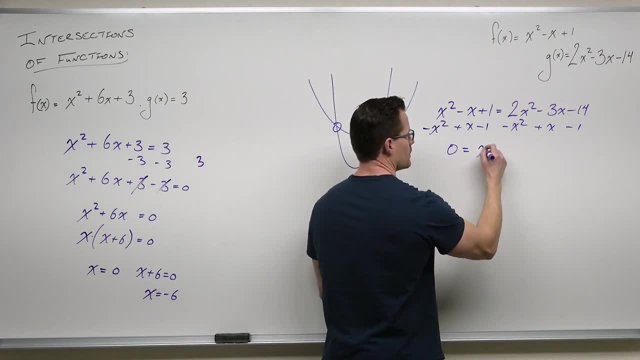 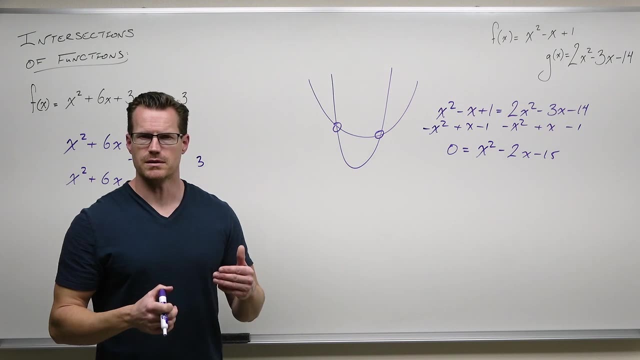 a quadratic formula is necessary. We need that 0. And it looks like this is going to factor. but I want to talk about what if it didn't? Square method's off the table here. We can't do that. We definitely don't want to do complete. 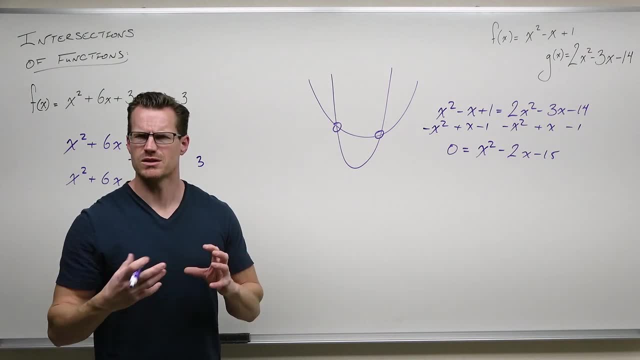 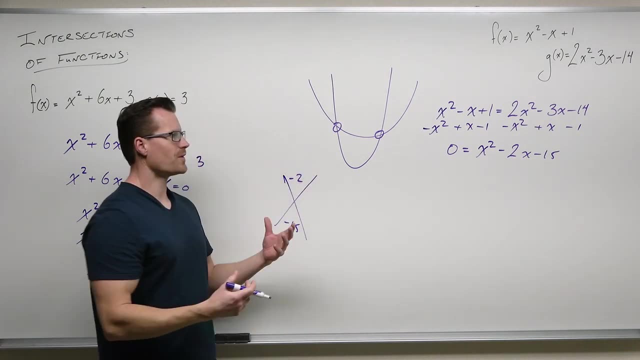 and square. We don't have to because we have some easier ways to go about doing that. So factoring would be number 1.. And we do know that this is going to factor because we can find some numbers that add to negative 2 and multiply to 1 times negative 15. That's going to be a positive. 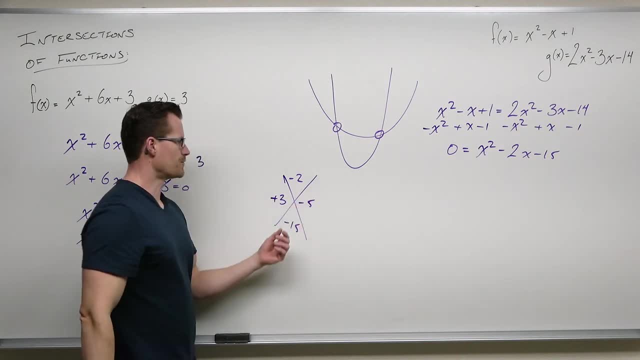 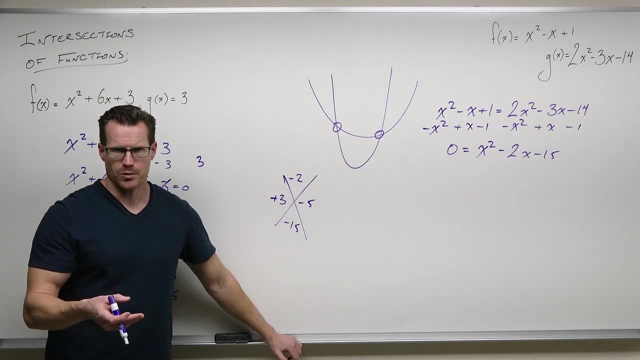 3 and a negative 5. That adds to negative. 2. That multiplies to negative 15. If that didn't work right now, you'd be doing the question quadratic formula And while you wouldn't find very nice values for your x- in this case x- 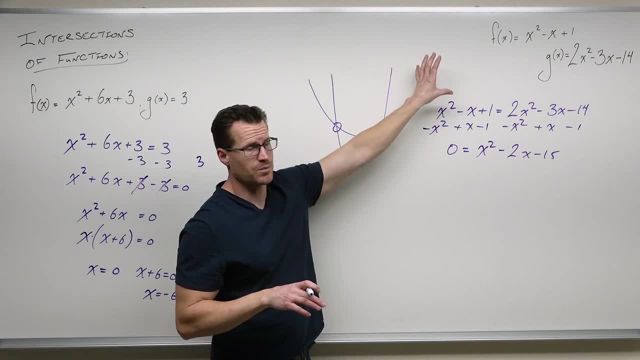 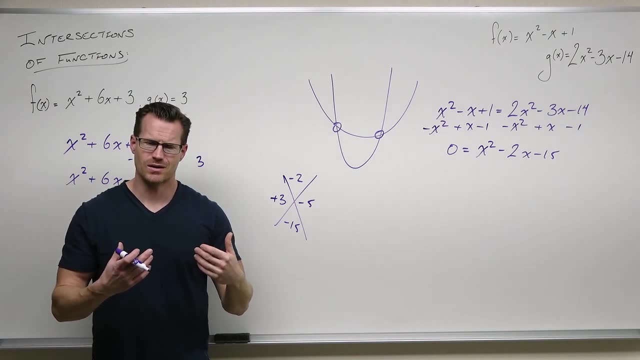 intercepts in what we're really in the context of the problem x, values of the points of intersection. they wouldn't be nice but they wouldn't be accurate. So the quadratic formula gives us things that are sort of hard to manipulate, but they are very important to be able. 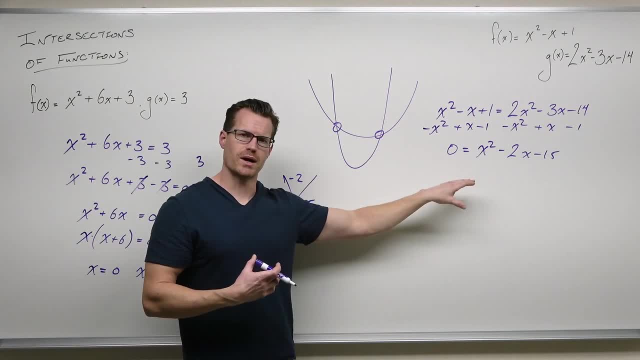 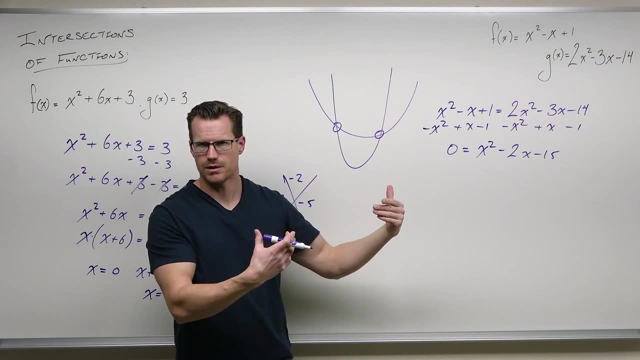 to find. So if this did not factor, you do quadratic formula right now and you'd have the x values from that of your points of intersection. What would be awkward is trying to plug them in and find output. That's where this would be awkward. That's why, most of the time, 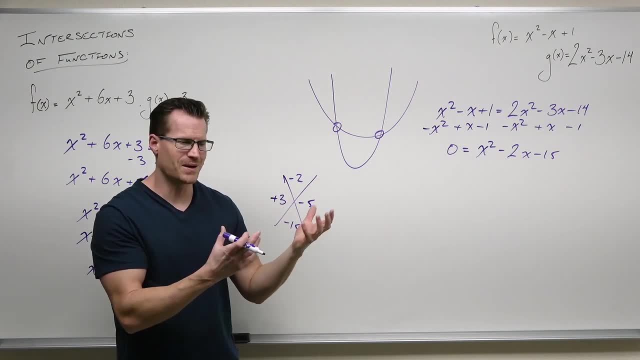 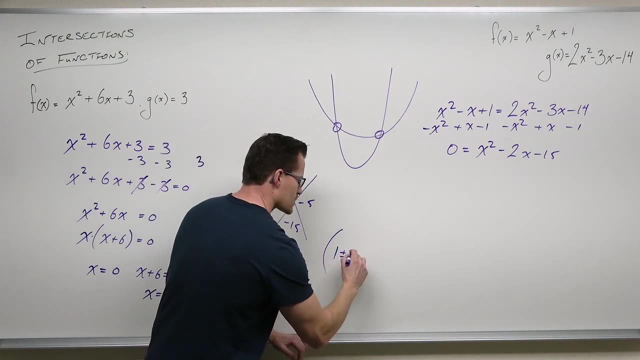 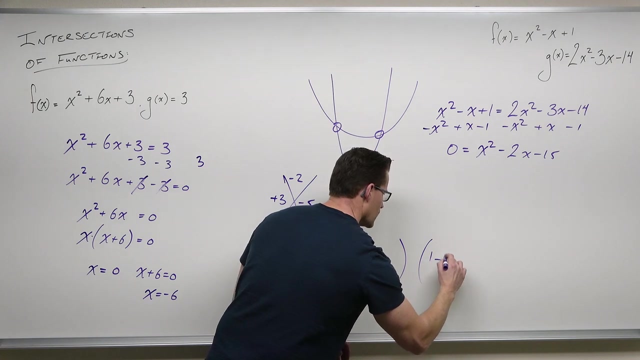 these things are factorable, so that you don't end with stuff from quadratic formula, Because can you imagine, I'm making this up. but I mean what if you had like 1 plus or minus square root of 3 over 1, plus square root of 3 over 2 and 1 minus square root of 3 over 2, something you could? 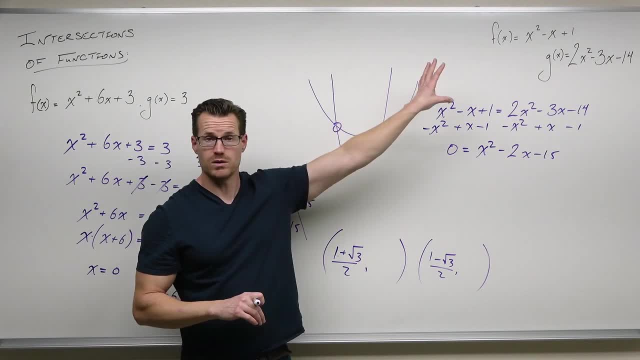 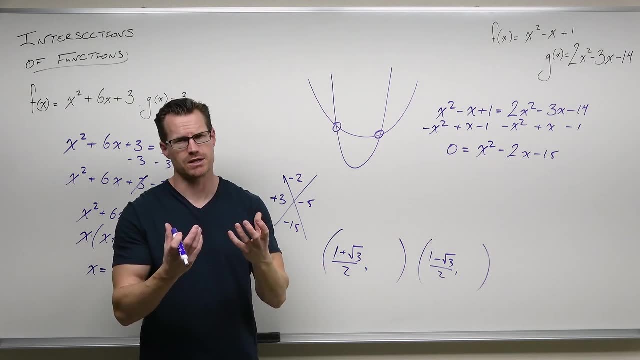 easily get from the quadratic formula. How would you plug that in? Well, you could do it, but it's going to be something very, very awkward for your y coordinate and we need to find ordered pairs or points of intersection. That's the whole idea. So that's why most of these are factorable is. 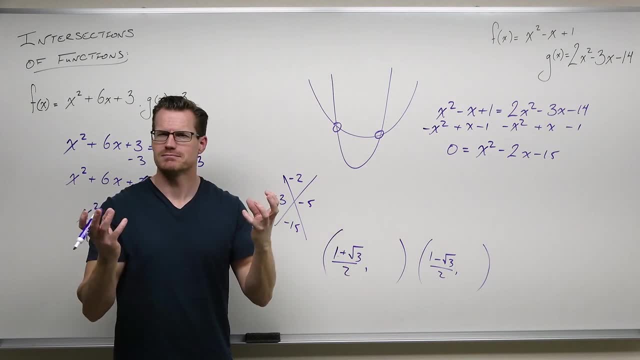 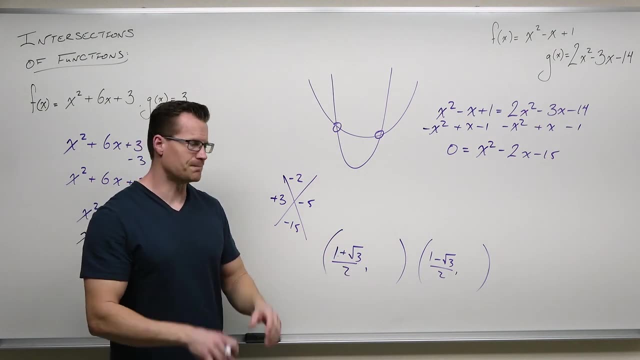 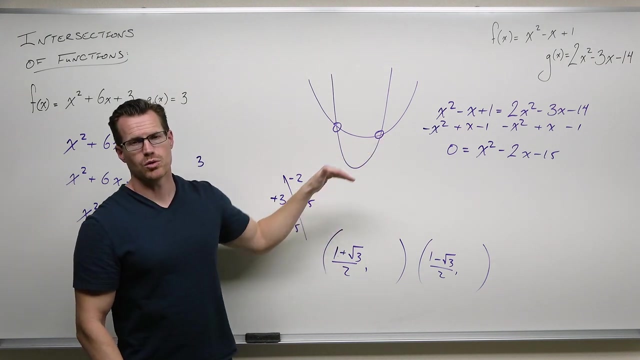 because you don't end with stuff that looks quadratic, formula-y, You don't end with stuff with radicals in it. essentially, if it's factorable, So again factor it. If it's not factorable, make sure you've really tried to factor it. If it's still not factorable, then do. 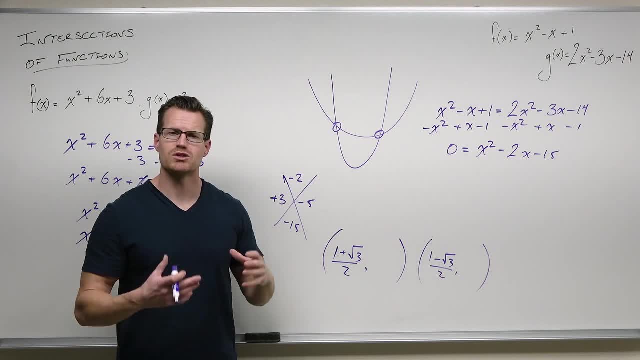 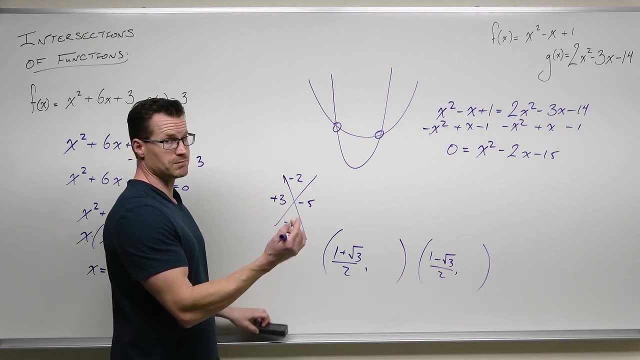 quadratic formula. You're going to end with some nasty values of your points of intersection, but plug them in anyway. Don't use approximations. You have to use exact values, unless they specifically tell you to use approximations. and then, of course, 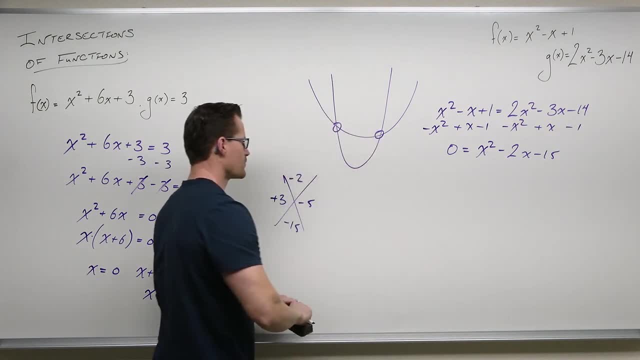 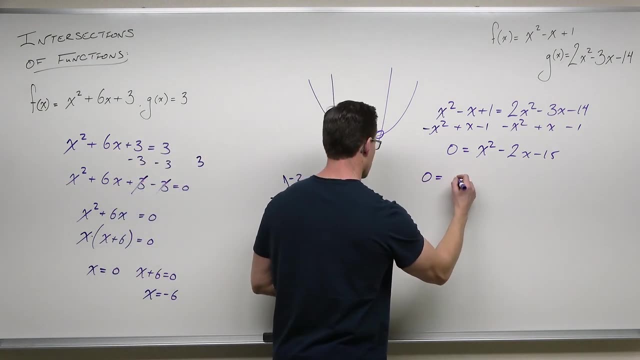 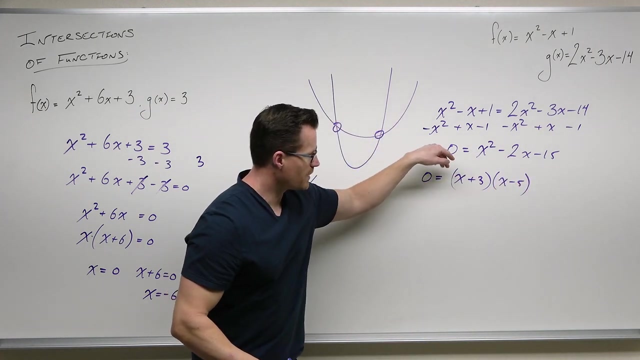 do it So for us. since this is factorable, we also know our a is 1,, which gives us something really nice. It's a great shortcut we can use. Maybe double check our work: x squared minus 5x plus 3x is minus 2x and then minus 15.. Set both of these equal to. 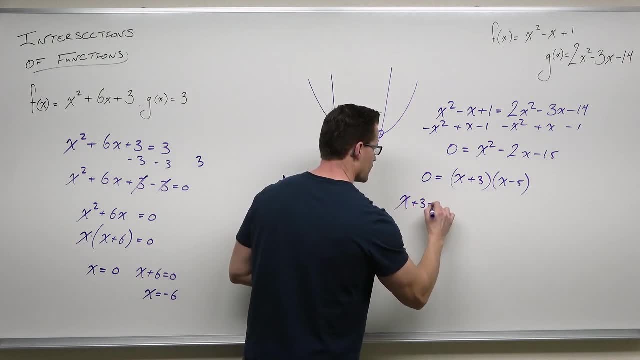 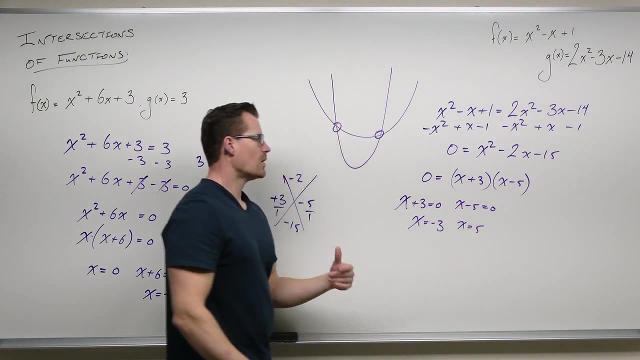 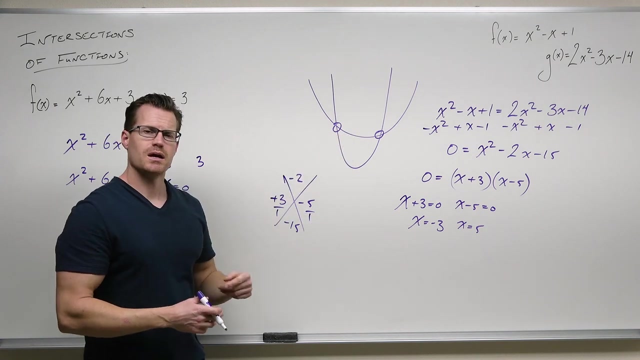 zero by the zero product property. And we now have the x coordinates of our points of intersection, of this parabola intersecting the other one. So basically, our x values are this and this. If we plug them in to our functions, evaluate our functions at these values, we'll find the 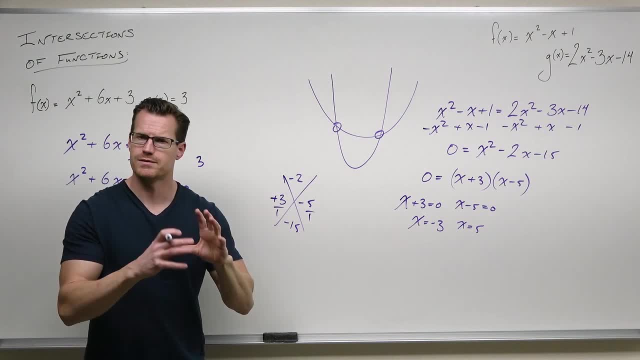 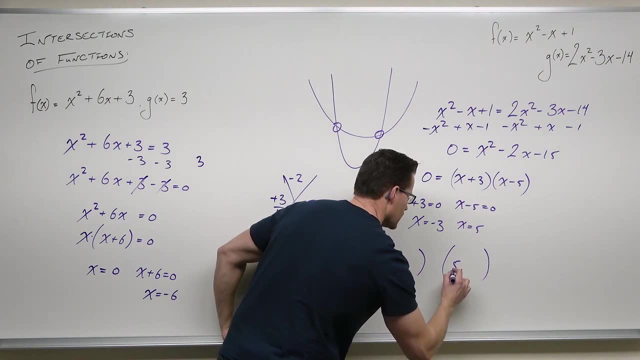 outputs. That's how functions work. Plug in the x, get down to y. That gives you an ordered pair. Also, we notice, man, if we just change these signs, we get the same values. You can. you can do. 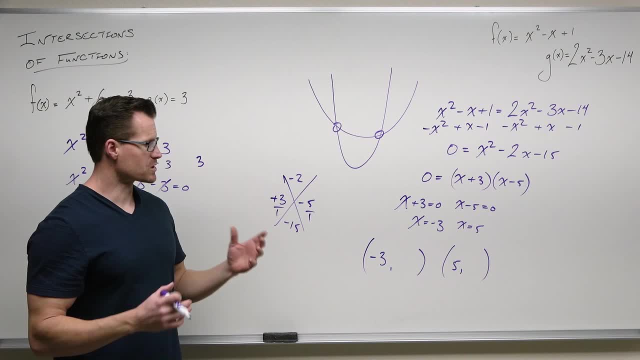 that. So let's take negative 3.. Let's plug this in. We're going to do both of them, just to make sure that we're right. So negative 3 squared. I'm looking at f of x. that gives you 9. 9 minus. 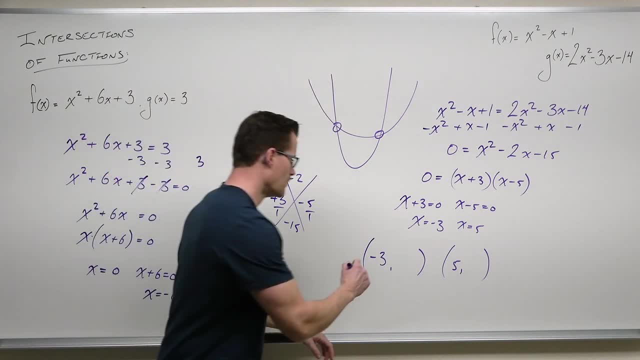 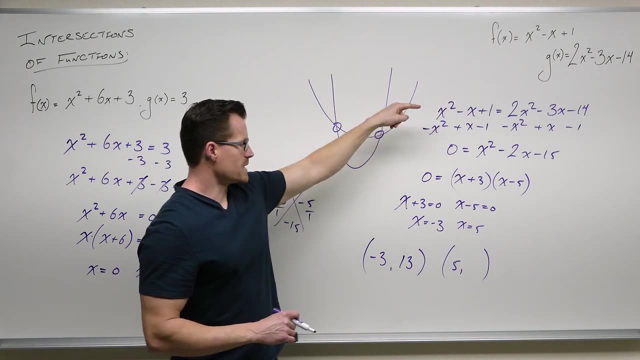 negative 3,, that's 9 plus 3, 12.. 12 plus 1 is 13.. I'm going to write it down, but I'm also going to check over here. So again, 3 squared is 9.. 9 times 2 is 18.. 18 plus 9 is 13.. So we're going to do. 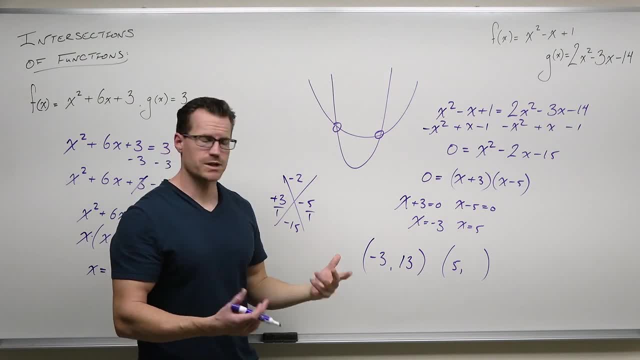 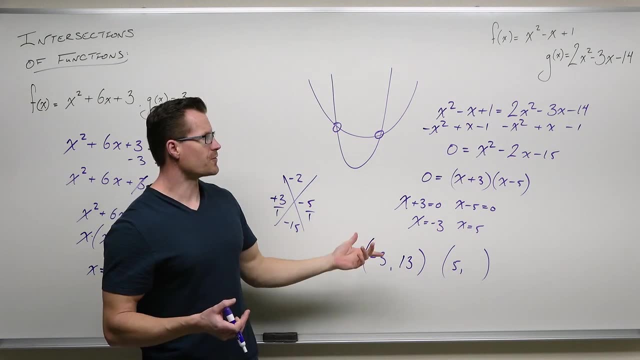 9 minus 9 is 27,, and 27 minus 14 is again 13.. So I know that this value of negative 3 in both of my functions gives me out 13.. That verifies that that is a point of intersection. Now the 5, same.